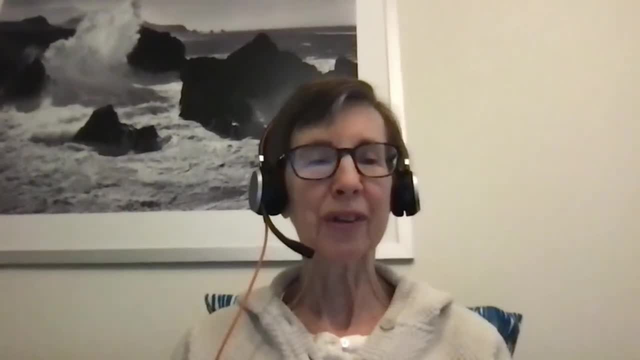 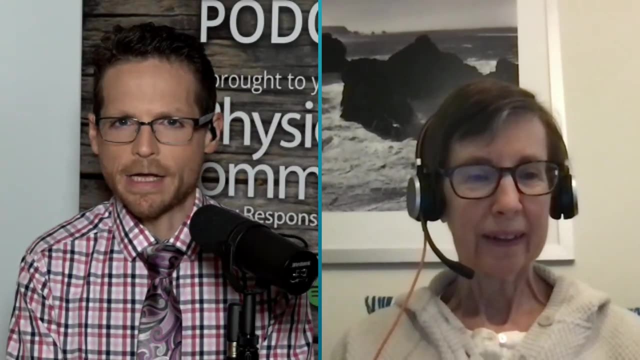 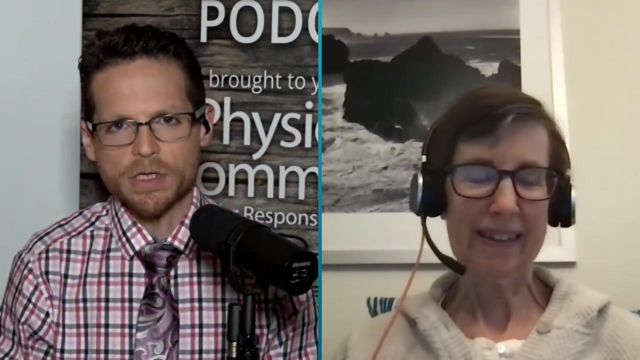 Western world, And so I switched at that point. All right, And nice to meet you, 1984,. I would imagine that there were not a whole lot of vegetarians in the world at that point. right, We hadn't seen that trend start to explode, as we're beginning to see now. 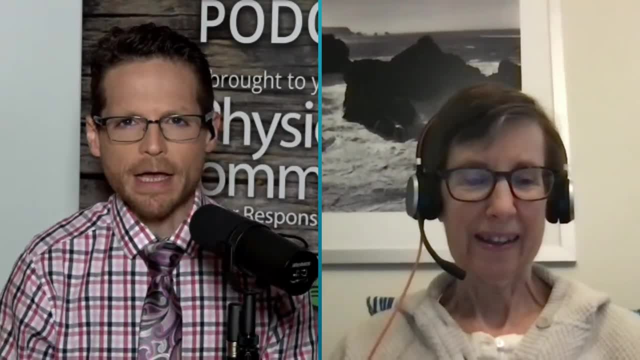 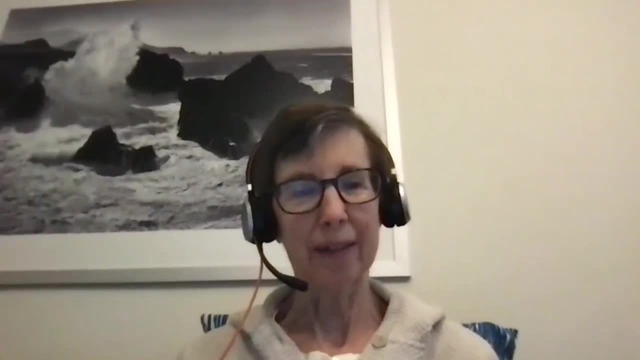 What kind of reaction did you get from your friends and your family at that point? Well, you're right, There weren't the products in the stores that you can buy to make cooking easy? It was, yeah, Well, I was just pretty. 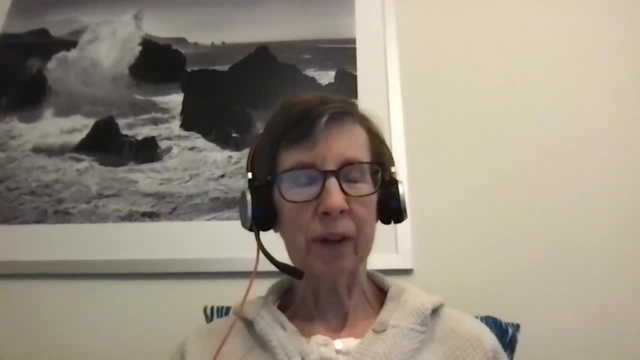 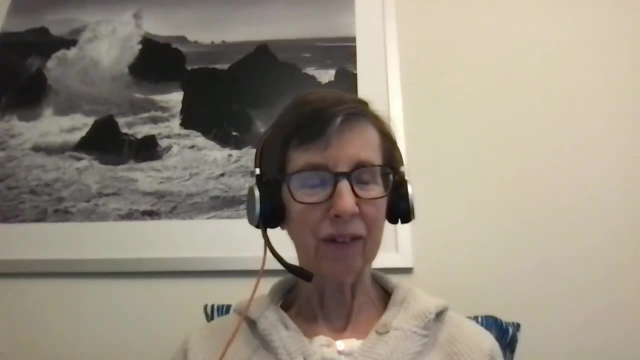 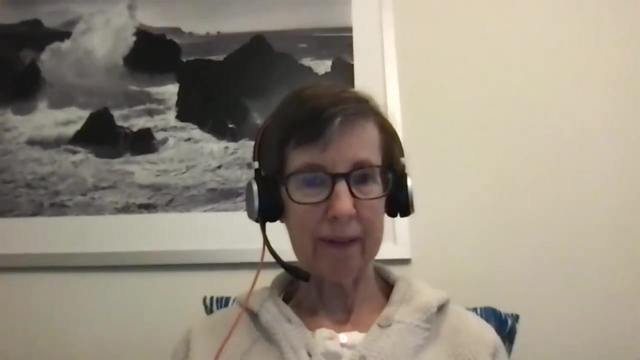 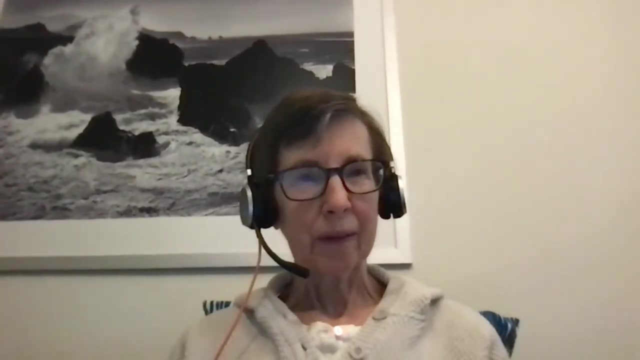 determined, And so I didn't really worry about my friends' reactions so much. The family did not join me, I just cooked my own stuff. I was able to make dishes for the kids, and then I would take mine out before I added the meat, And then so for about three or four years. we kind of went our separate ways. And then my daughter, when she was seven, read a book about veterinarians And his daughter who loved animals so much she wouldn't eat them. And so then my daughter became vegetarian at age seven. So then there was my daughter and I eating vegetarian, and then my husband and two sons were 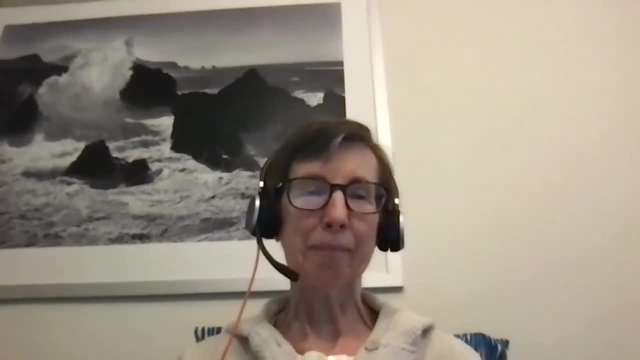 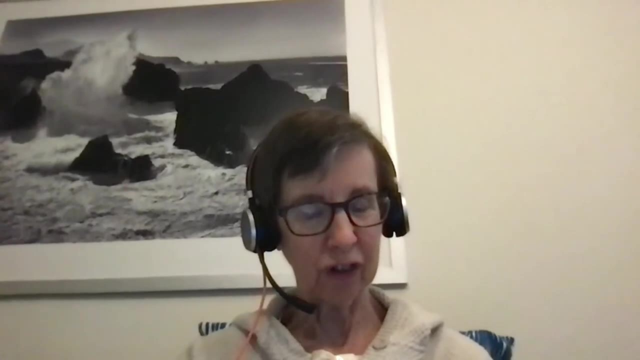 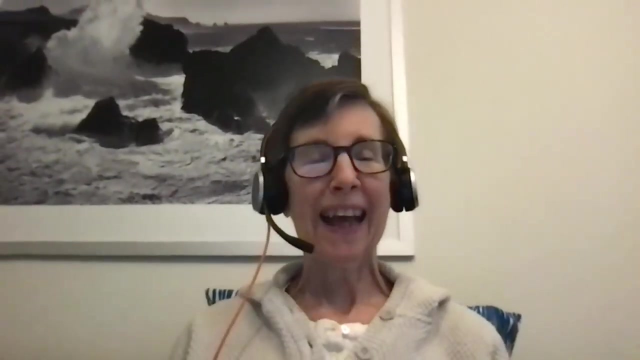 not, But over the years my son had to do a paper for school and he contrasted Guandi and Churchill. He read about Gundy's Ahimsa philosophy and he became vegetarian Then, as my husband, as a physician, learned more and more about the health impacts of red meat. he left that off And then he got rid of chicken so he became vegetarian. And finally our middle son. We were on a trip to California driving past stockyards And he said later: it was so difficult being in the car with four vegetarians driving past stockyards that he, he also became vegetarian. So it took eight years, but then we were finally all in the same place. 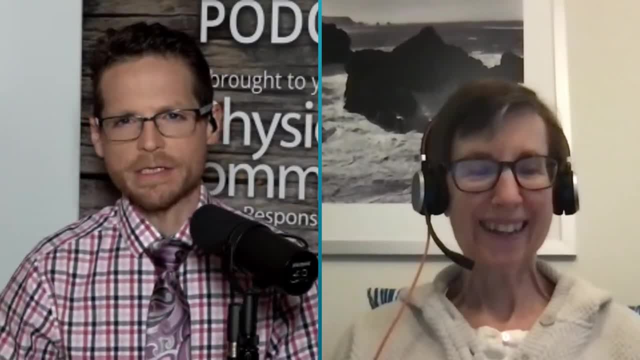 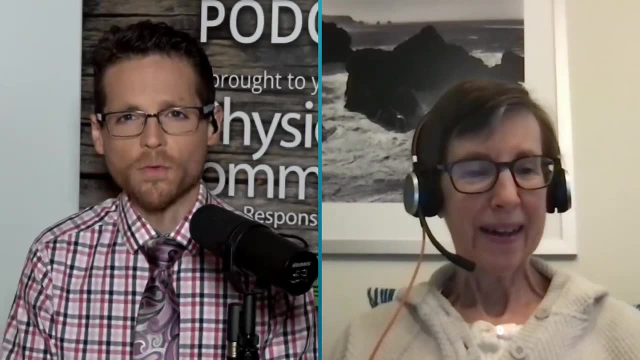 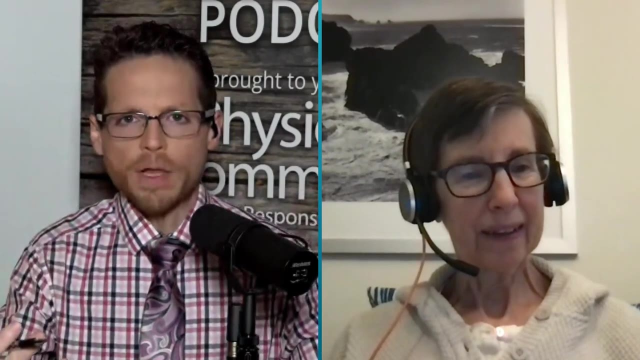 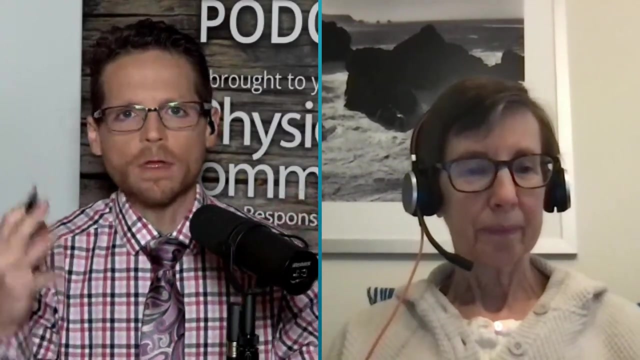 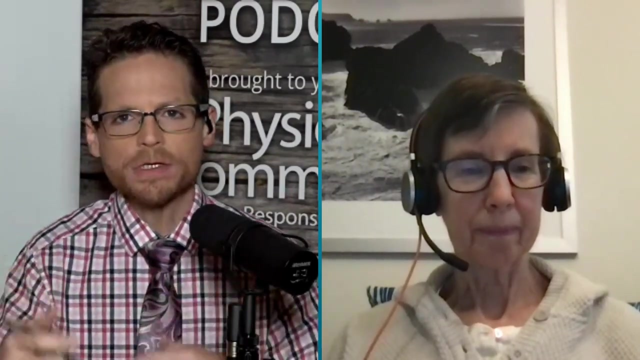 So eight years from 1984. I'm guessing this is right around 1992 at that point, right, Right, right. Okay, now let me let me pause before we move forward with your story, Because one of the questions that we get all the time on the show, Jean, is: I am new to this plant based diet, but my family has not joined me on this journey, So I'm finding it really difficult to cook two meals every single time. How did you balance that? How did you make that happen? Are there any tips that you can share? 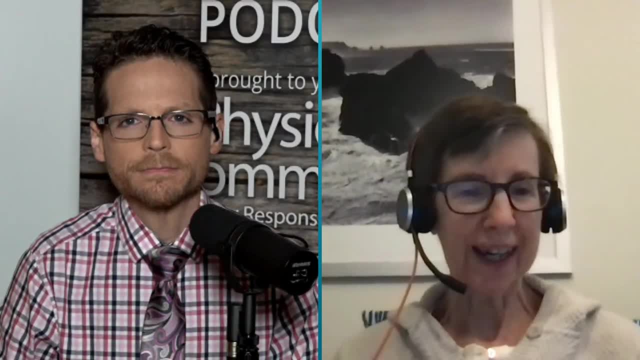 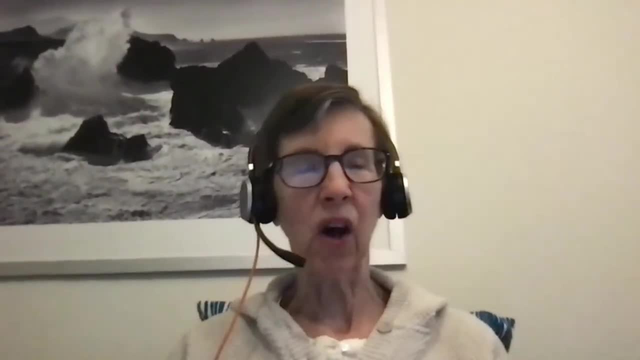 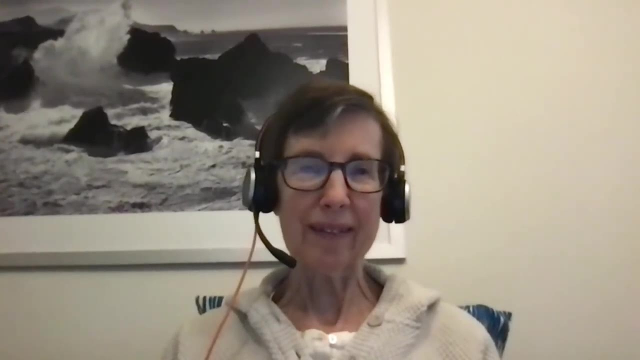 Well, I looked for recipes where you add the meat later, You know, and or it was just a separate thing, And I ate all the side dishes and made sure that I had beans in something. So it really wasn't. it didn't seem that hard to me. 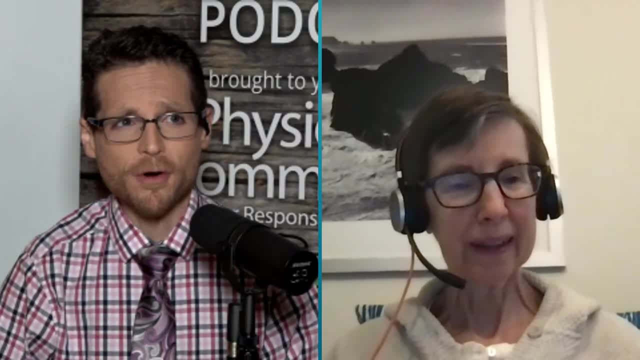 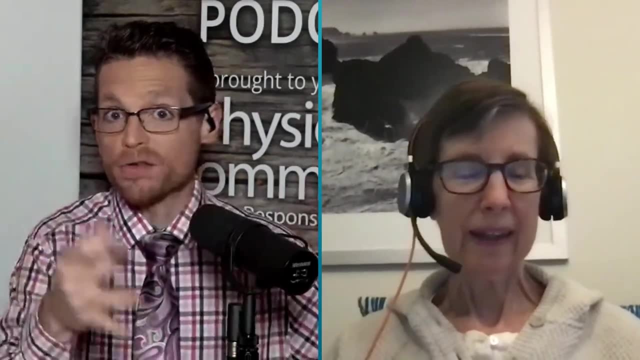 That is sage advice. That is the first time I think I've ever heard it like that. Like most people assume that you you have to do two different recipes, Like if you're doing meatloaf, you got to do the meatloaf and then you've got to do the lentil loaf. 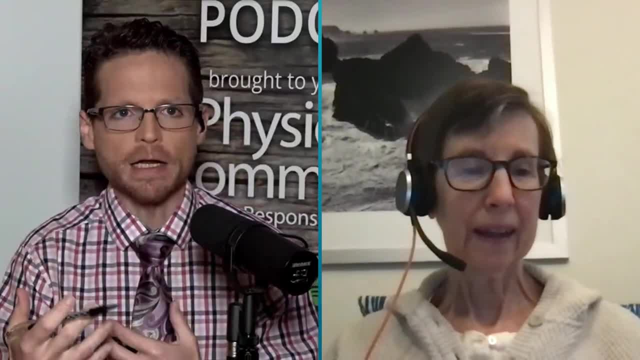 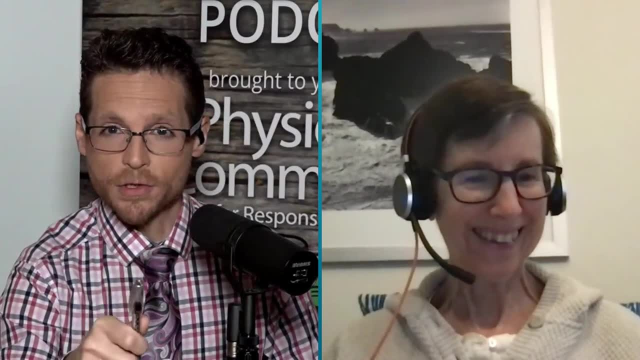 And then you've got to go with it, Right, But now you're talking about just being smart about it and adding the non-vegan products down the line. I like where your head's at, Jean. This is why I have you on the show, because you are bringing a ton of wisdom to us. Let's flash forward another five years. 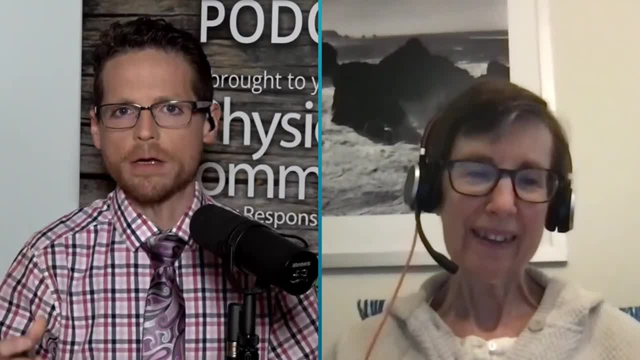 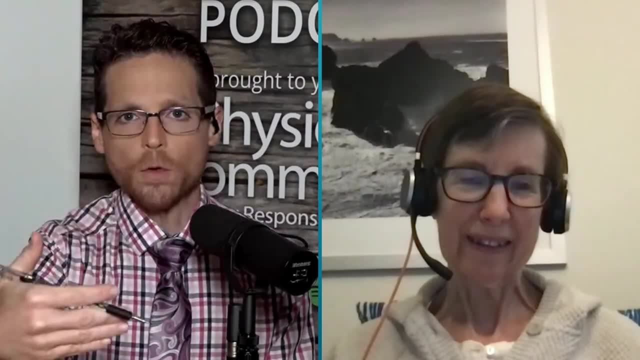 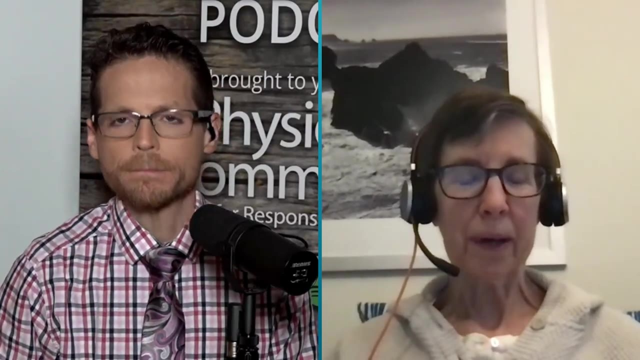 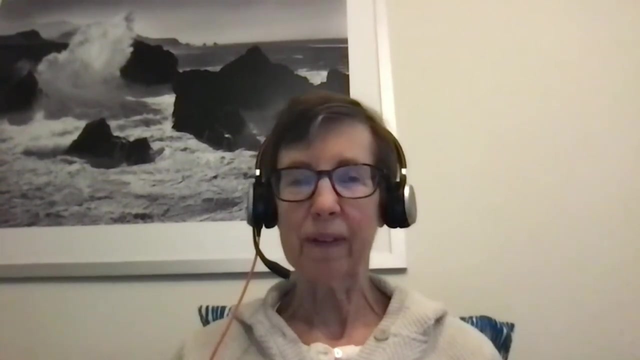 1997 for you was another big year. That's when you decided that you didn't just want to be vegetarian, You wanted to become a full-blown vegan. at that point, What was the deciding factor there? That was learning more about the egg and dairy industries and what happens Before that. I just had never heard that all these baby chicks were killed. The male chicks were killed. I didn't know that. 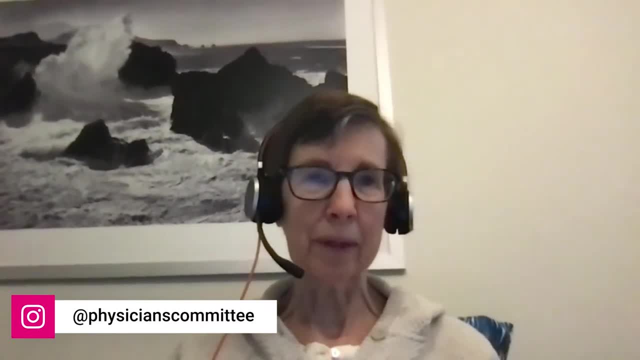 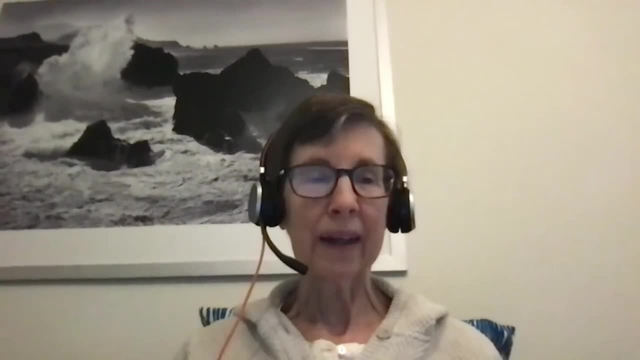 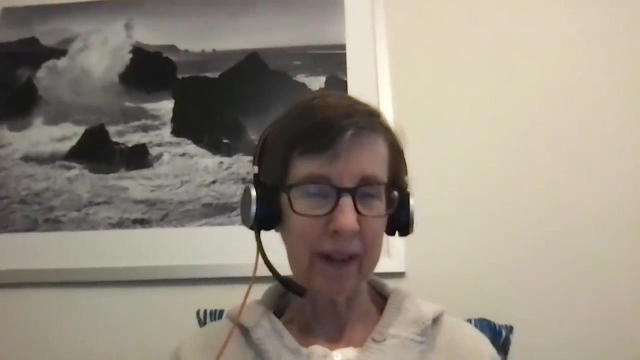 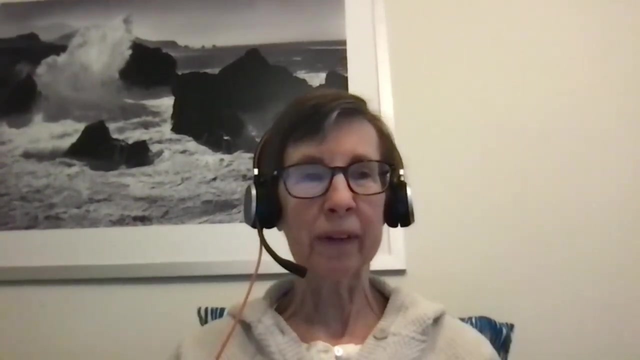 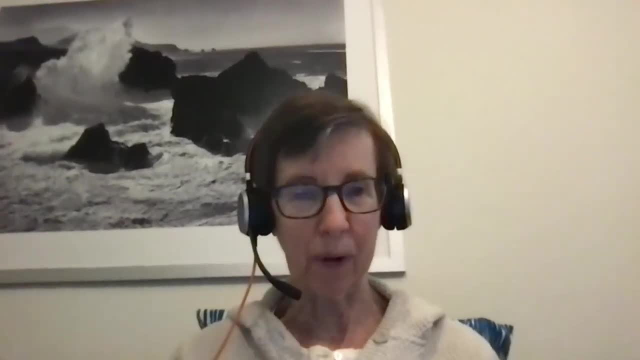 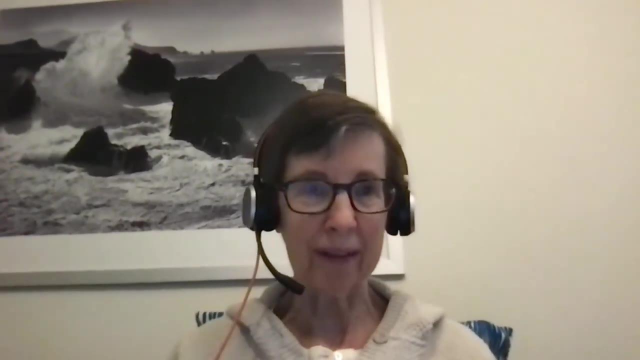 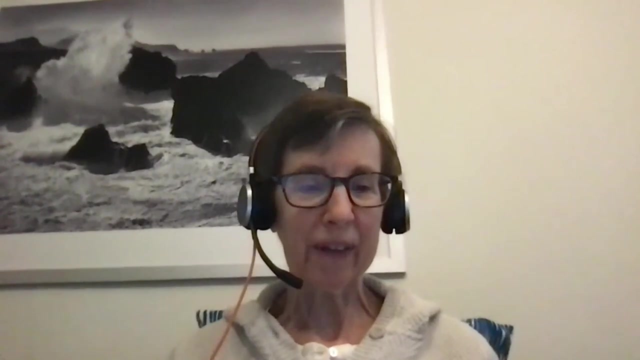 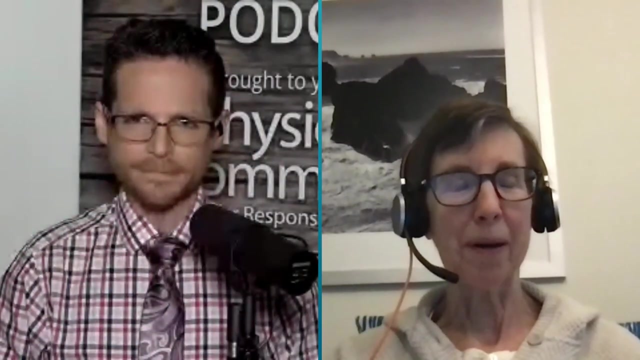 I just got it in my brain that anytime I wanted dairy I would think of the cow. You know cows have a gestation period as long as humans, you know, and they mourn for their calves when they're taken away. So you know, that just really touched me And you know I had been a nursing mom, so I know about motherhood. 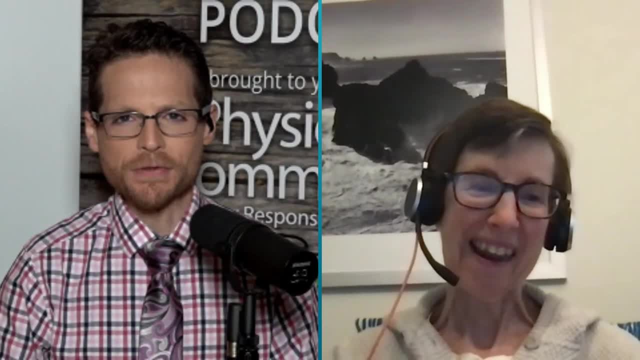 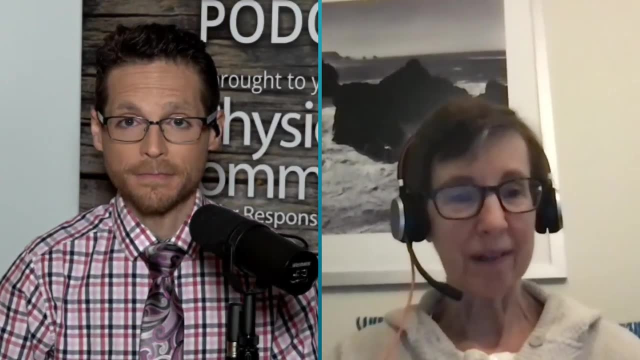 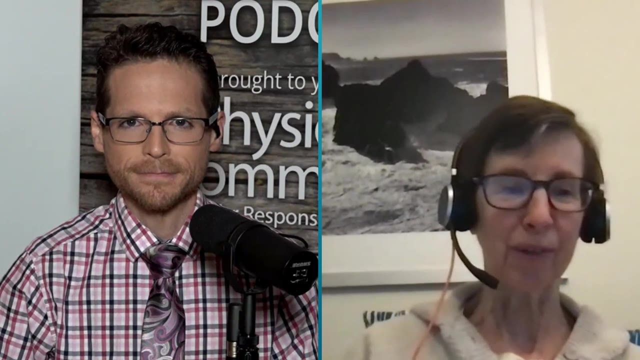 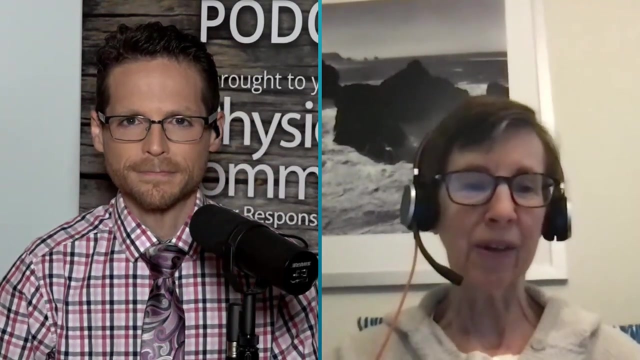 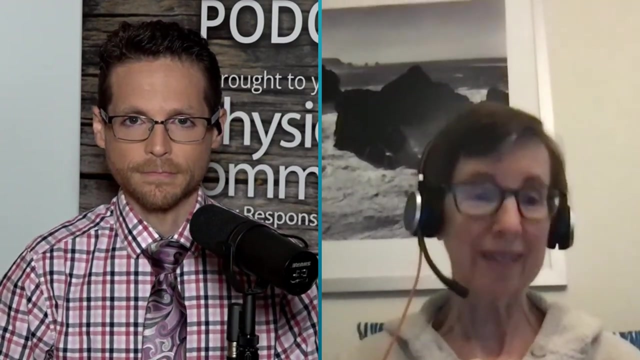 You mentioned that frozen yogurt was hard Struggled with cheese. Was that a big one for you? It wasn't as big for me as it was for my husband. He really struggled with cheese And for several years we didn't have any at home. But if we went to a party or something, you know he might have a little bit. But it takes a while to lose that addiction And I think Neil has done such a great job, you know, in his books and his talks about informing people that cheese is an addiction. 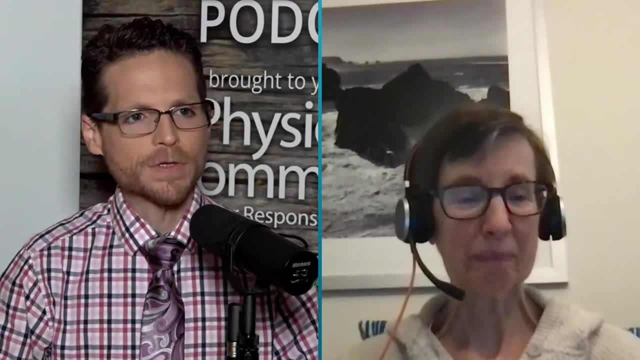 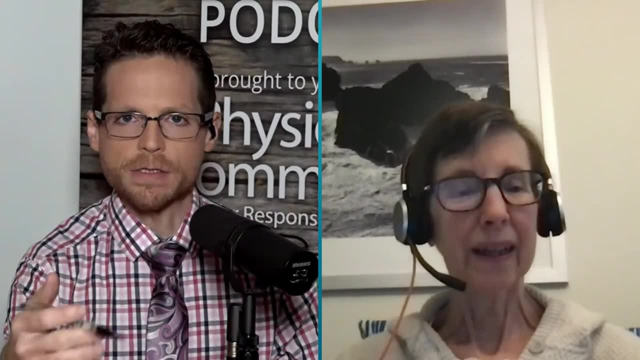 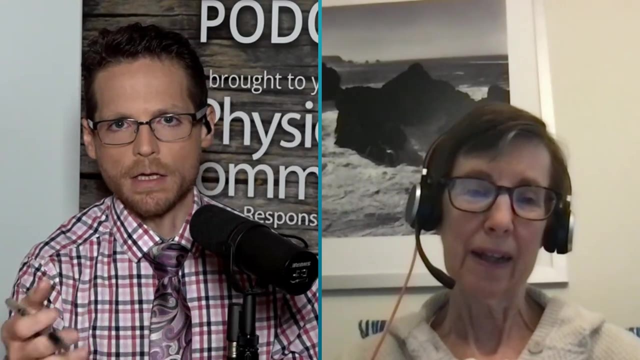 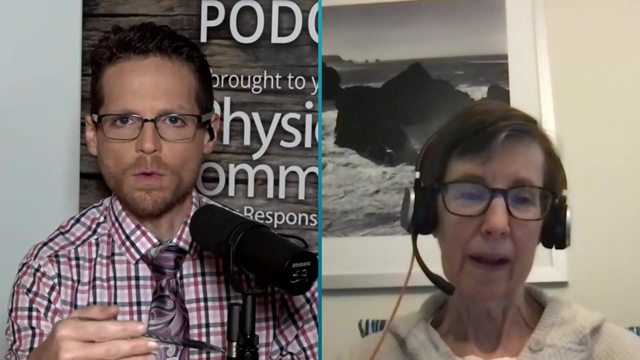 Yeah Yeah, The Cheese Trap is a great book. Yes, So your husband, the physician. he goes primarily for health reasons. That's his big deciding factor for changing up his diet. You, it seems more you're on the animal side and the environment side We'll get into that as well. But how important were the health benefits to you while you're making all of these decisions as well? 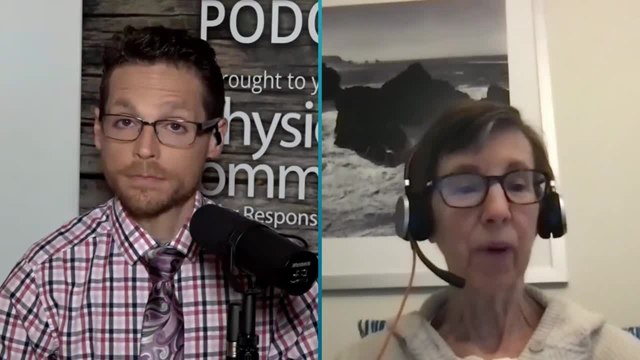 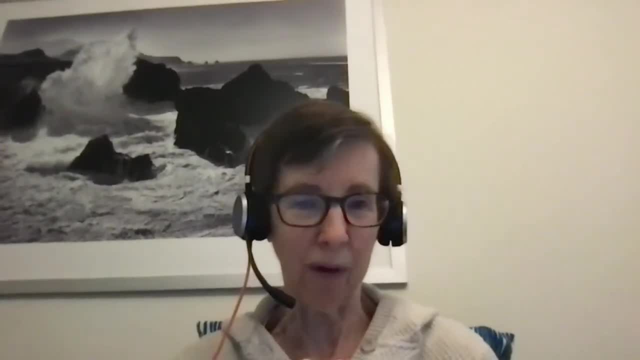 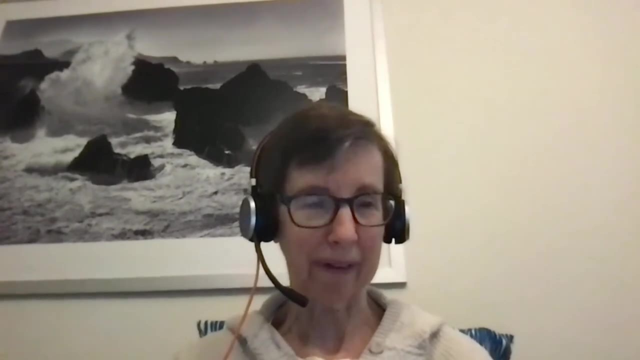 Well, I always felt pretty healthy. What I was supposed I was surprised by, though. I always had a sinus infection every winter and just figured you know, that's normal, You get a cold and it turns into a sinus infection. But after I gave up dairy I didn't have another one ever, So that was pretty surprising, because that's not something a lot of people know. I did not realize. Man, that's fantastic. So getting rid of the dairy seemed to cure your sinus ales. Yes, Right down to the infection. Well, that's got to be a pleasant surprise. That must have been a nice winter, the first time you went through all of those cold weather months and didn't get sick. 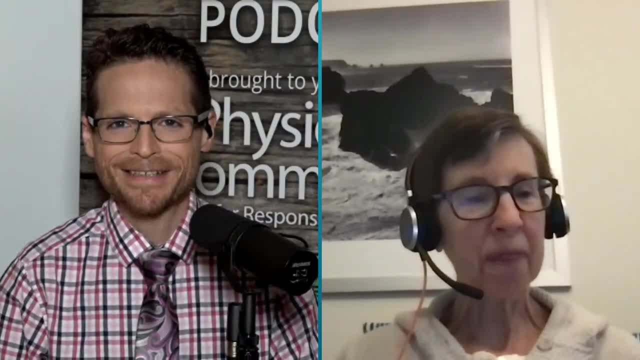 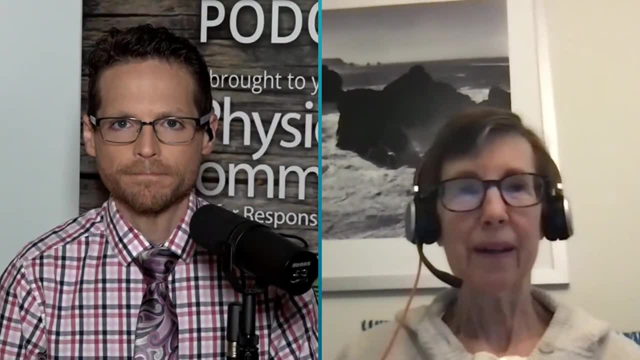 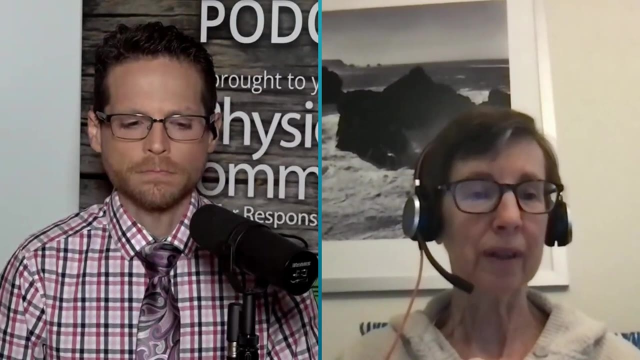 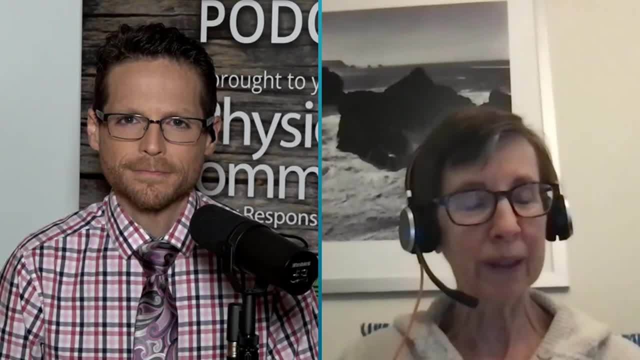 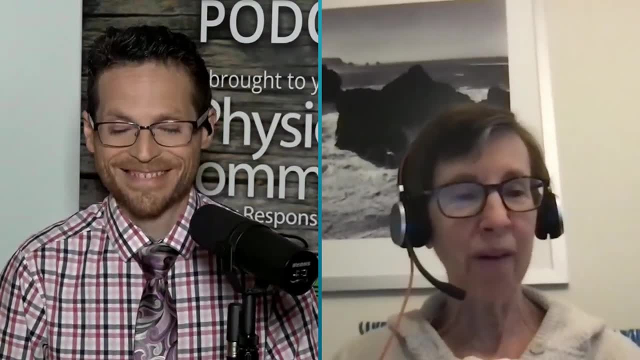 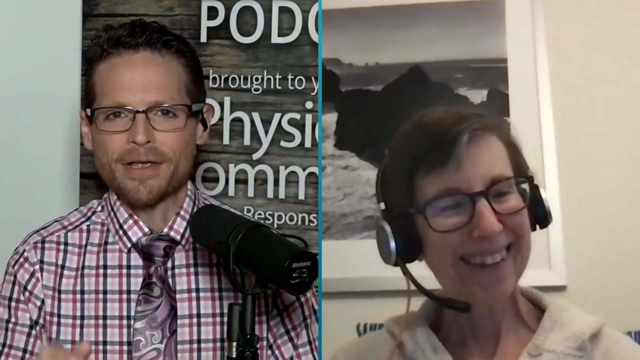 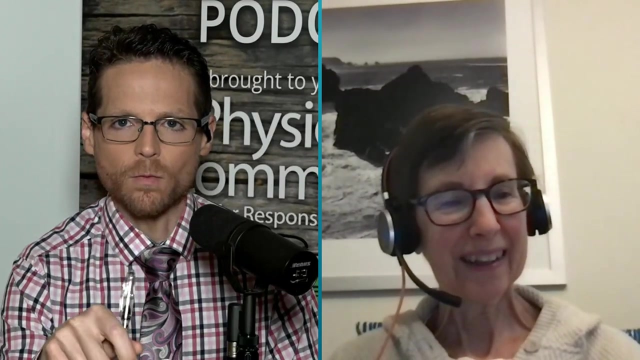 Right, Right Now you're in my wheelhouse talking about struggling with your weight, So let's, let's spend a little bit of time talking about that. What were some of the foods, beyond just the cheesecake, that you were really attracted to? 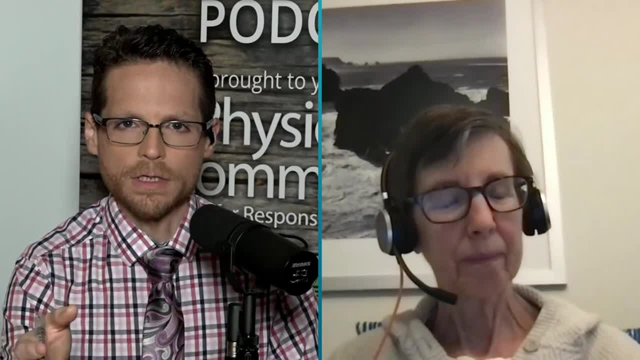 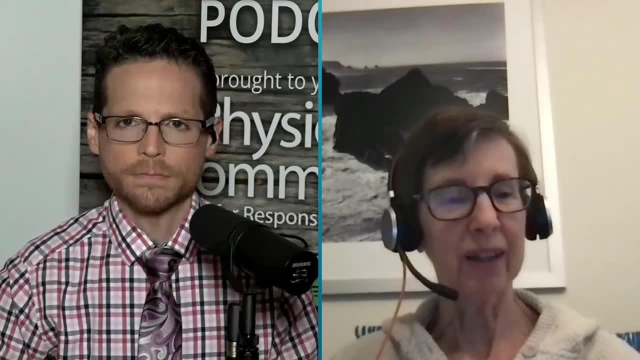 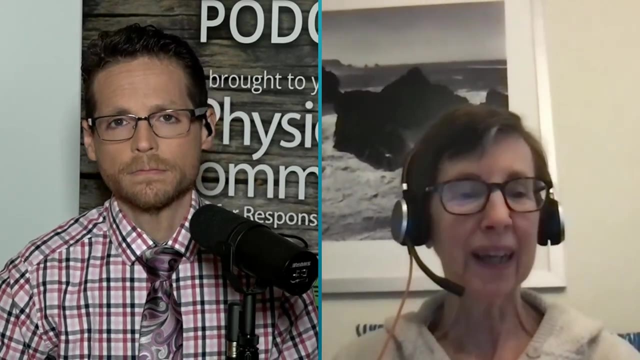 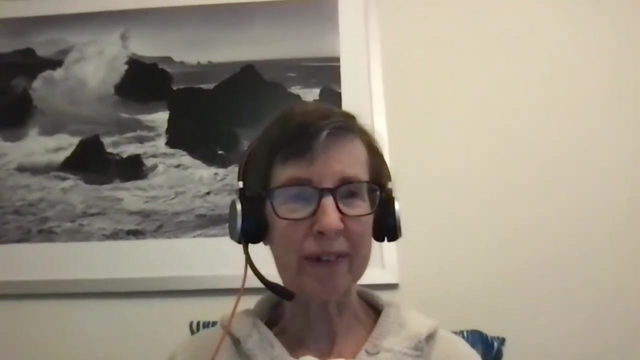 really attracted to during your teens and early 20s? Well, I was attracted to junk food. I was a binger on junk food, You know. you get a bag of whatever kind of snacks and I would just eat the whole thing. At that point I was working three to 11 as a nurse in the hospital and you come home. 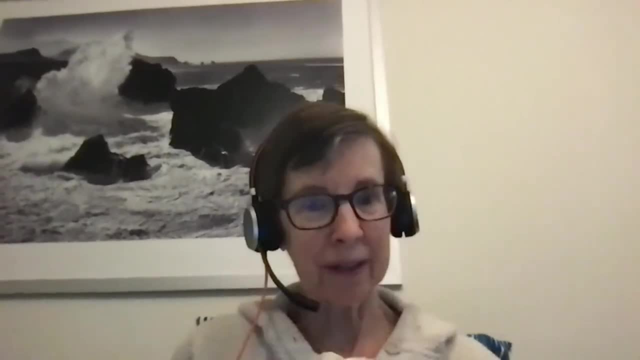 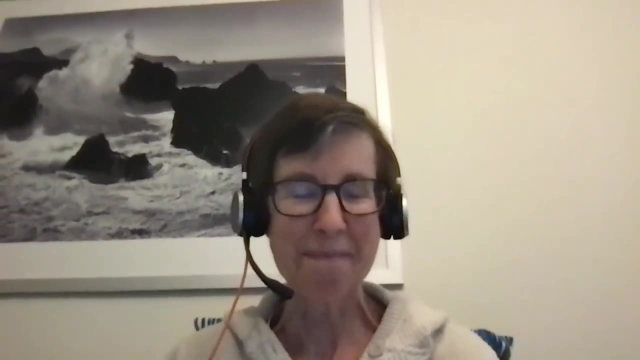 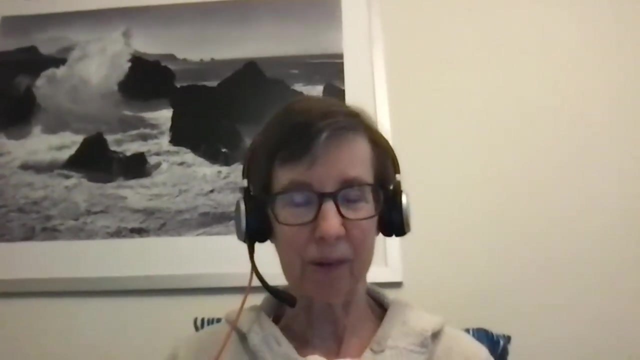 at 11 and you're exhausted, but you can't unwind yet to go to sleep, And so I would eat, And you may know, nighttime eating is not a good time, And so just the whole lifestyle. And then you know, I would try every diet that came out. I went on the Atkins diet before it was called that It was. 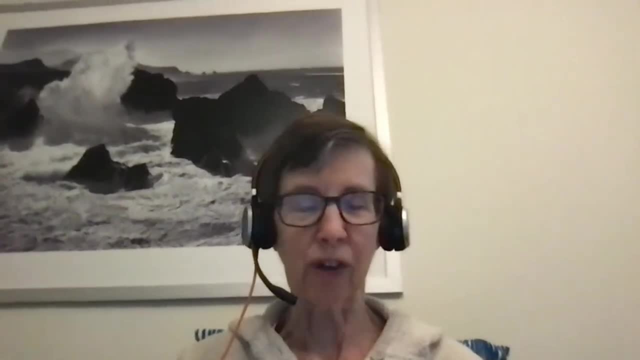 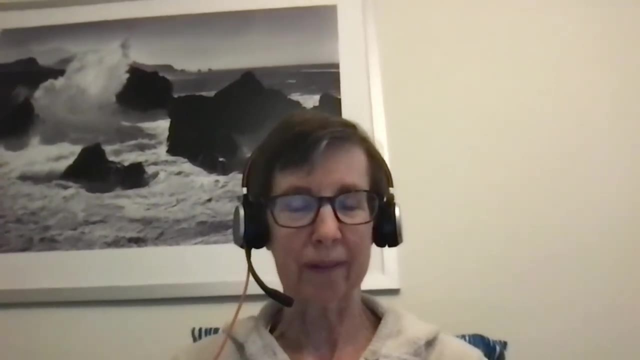 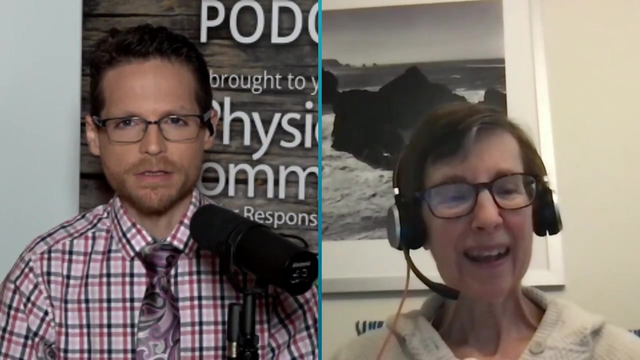 Dr Stillman's weight loss diet in high school. I tried that- total protein, nothing else, And I got so sick that, fortunately, I quit it after two weeks. Just two weeks and you were tapping out already. huh, Yeah, Oh man, Were you just getting nauseous or just generally not? I felt weak and 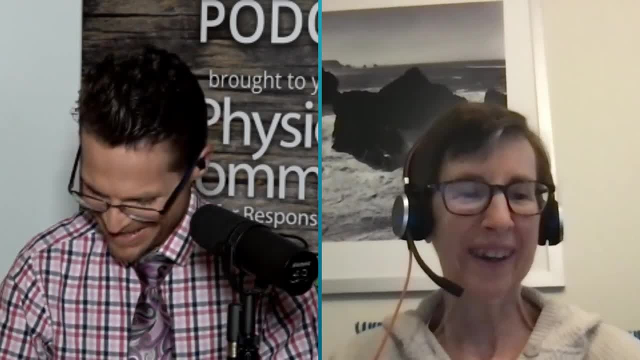 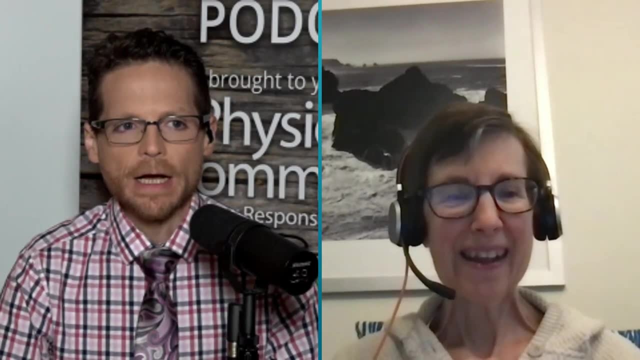 sick and I just couldn't look at cottage cheese again, you know. So it's interesting that you were a nurse working that three to 11 shift. A lot of times when we do the live shows on Wednesday, when we have a doctor on, people will ask: well, look, you know, I'm. 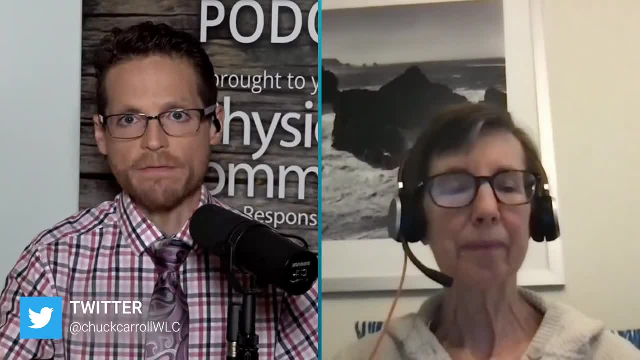 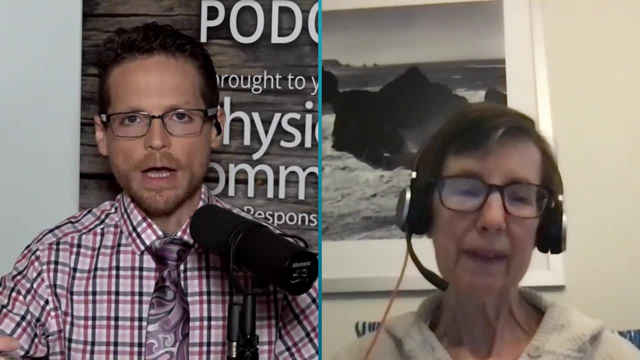 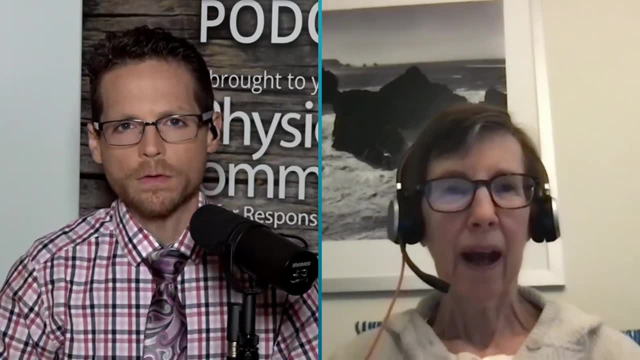 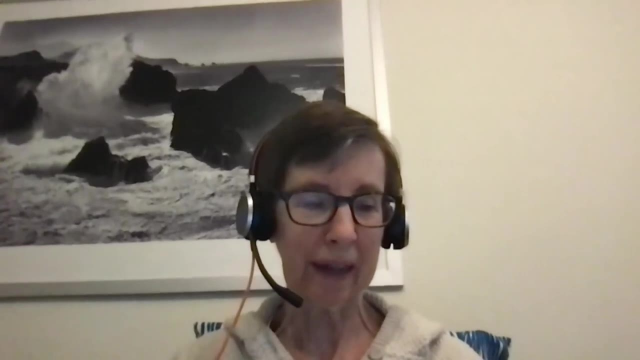 healthy when I'm keeping those hours. So what? what were some of the other tips, some other things that you eventually found that worked for you? Well, I have to say, I didn't stay with nursing and then that schedule, And I think that was one thing that helped. The other thing that 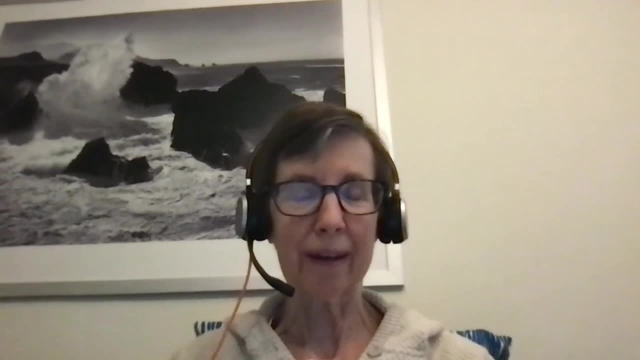 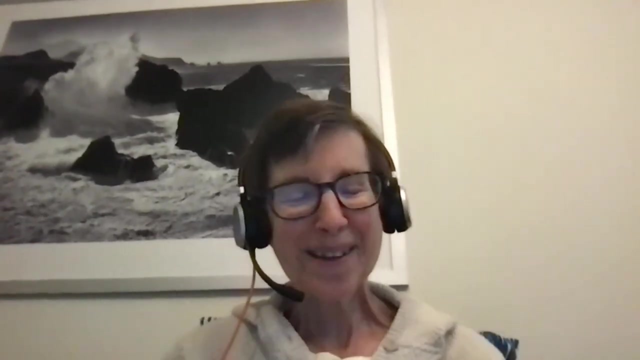 was most helpful to me, which is quite unusual- is getting pregnant. We had our first child and all of a sudden I read everything. It dawned on me that everything I ate was going into this baby. So I couldn't eat junk food Somehow. for myself I didn't care, but for the baby I cared. 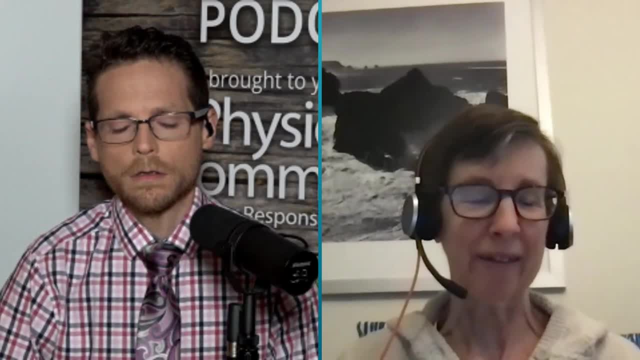 And so I quit junk food and that got it out of my life. Why do you think you had that philosophy when there's still this theory that you're not going to be able to eat junk food? Well, I think there's still this theory that you're not going to be able to eat junk food. out there that when you're pregnant and you have these cravings, you can basically eat whatever it is that you want. Ah well, what I read and what hit me was: I am creating a new life that depends on what I put in my body, And I don't want this poor baby to be suffering because they 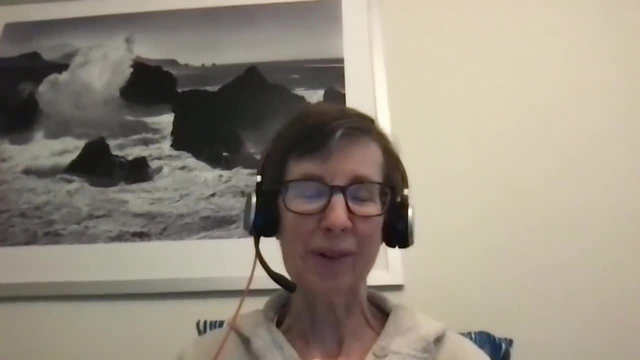 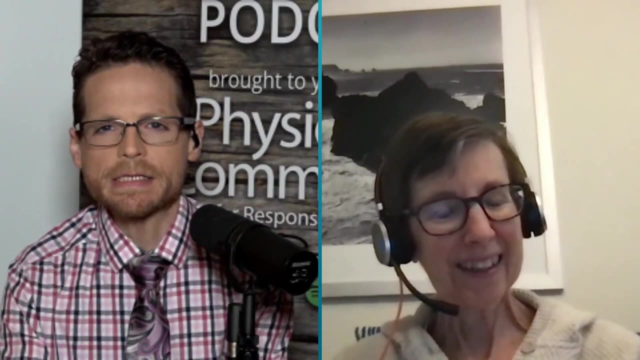 didn't have, you know, the antioxidants and the vitamins and minerals, and and junk food doesn't have that. Indeed, it does not. Um, okay, So we're back 1997 here. Uh, you're eating an exclusively plant-based diet, Um, and. 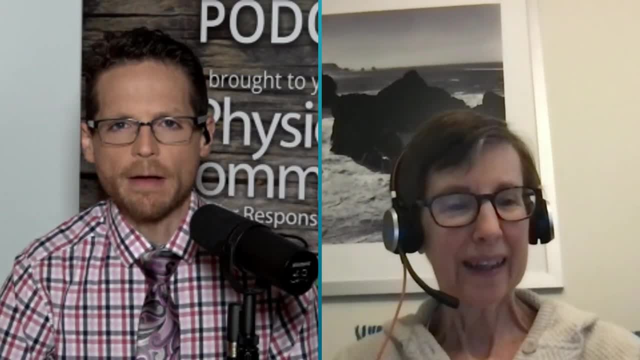 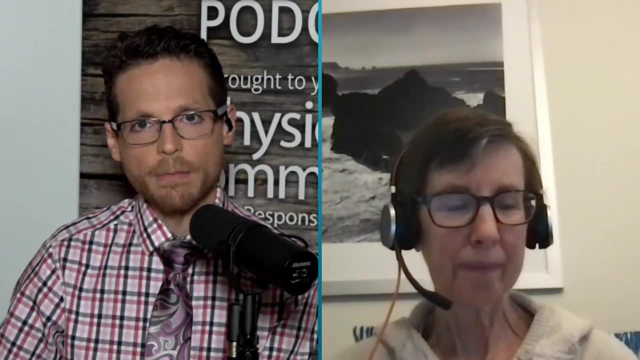 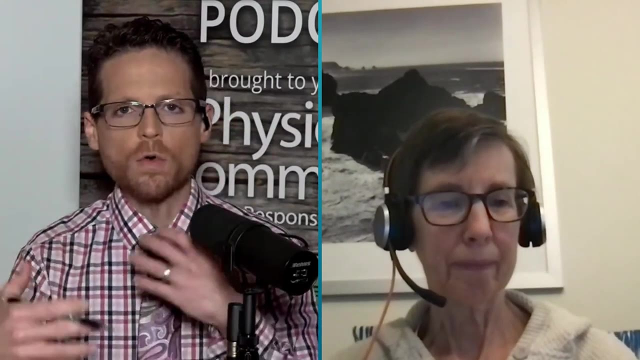 with this being such a momentous year for the food for life program. I'm guessing that because you eventually landed there, um, from 1997, from the time that you became an instructor, you just began to learn more and more and more about the benefits of plant-based eating. So what was getting you so? 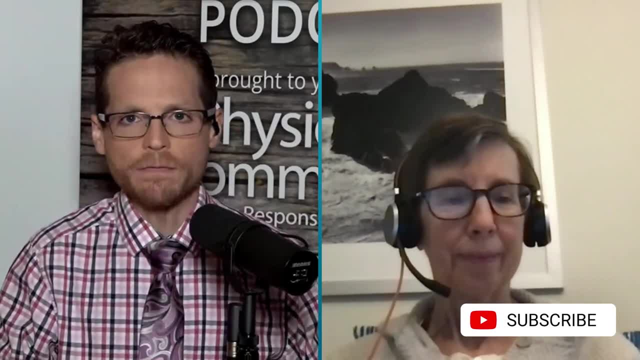 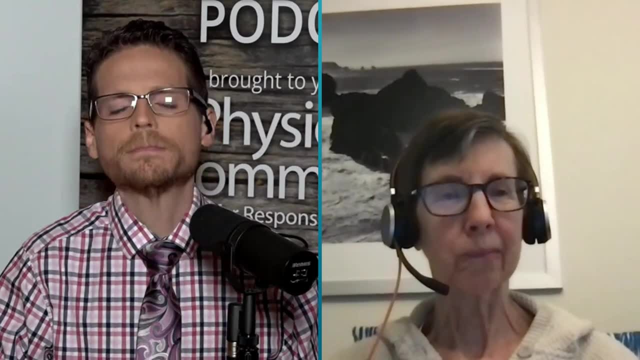 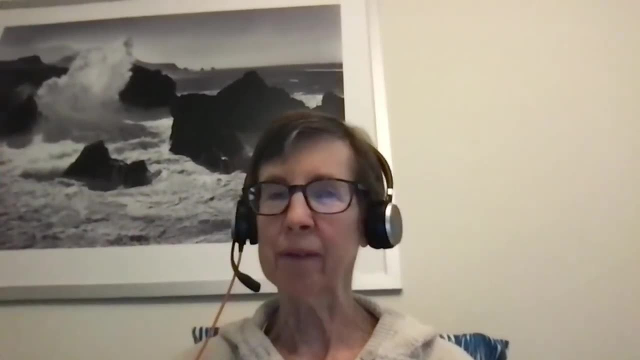 excited and so motivated to eventually become a food for life. Well, um, we were in Arizona in um, well, not 97, but when we, I joined PCRM fairly early because I remember getting their emails and you know their, their information, uh the uh. 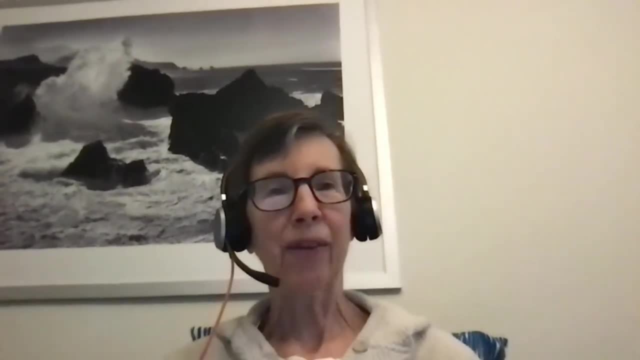 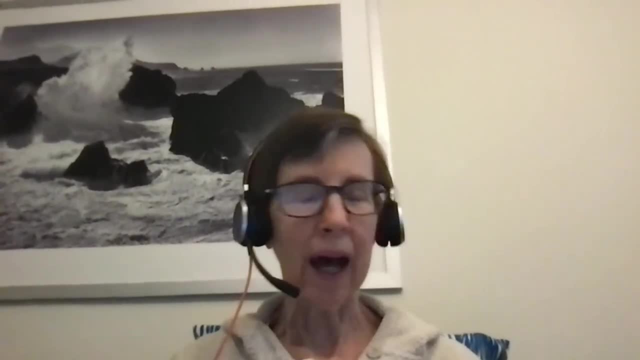 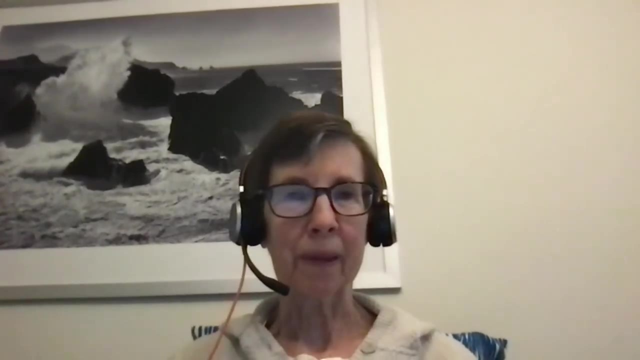 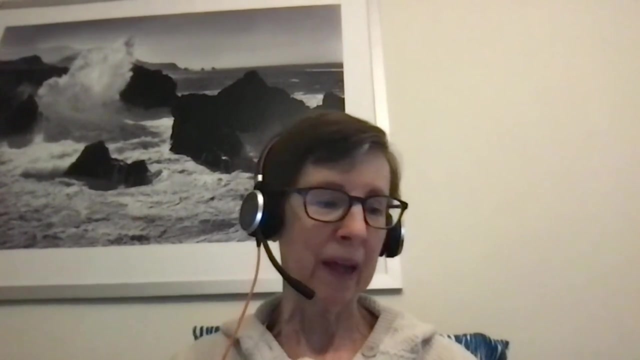 I heard about the food for life program for a while And then I was in a transition. I was, at that point, a marriage and family therapist in Arizona And, um, when I heard about the food for life, it just sounded so fun because I have always enjoyed cooking. Um, and I did have the 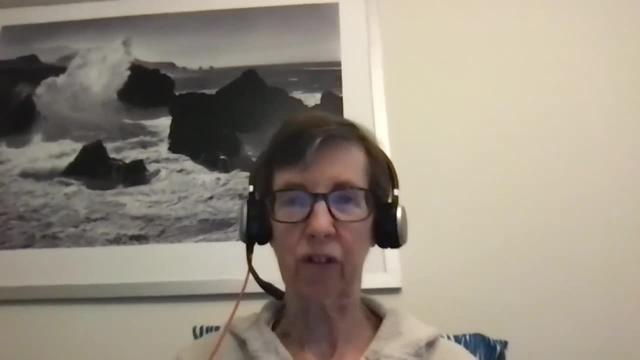 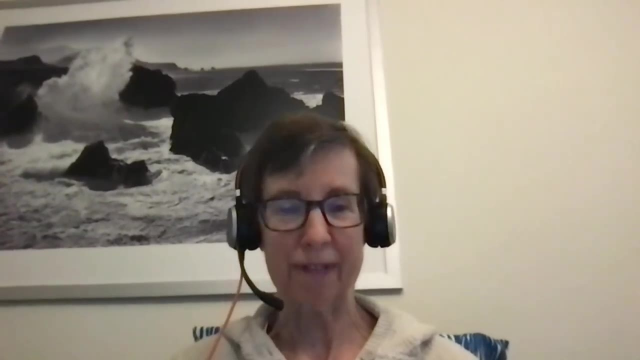 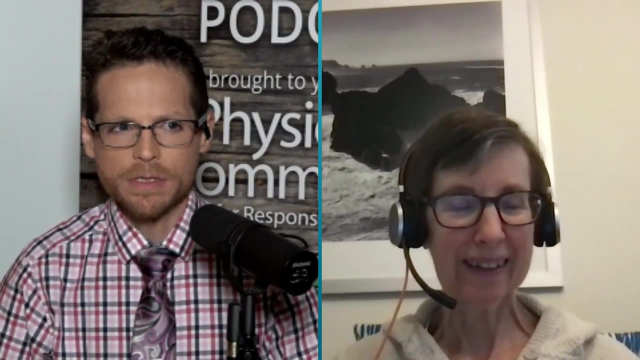 health background. at that time, you had to have a health background or a chef background, And, um, so I had the health background and I'll be able to cook. And I thought, wow, this sounds really fun. And that's what it turned out to be. Um, how, how was, uh, how was the class instruction for you? 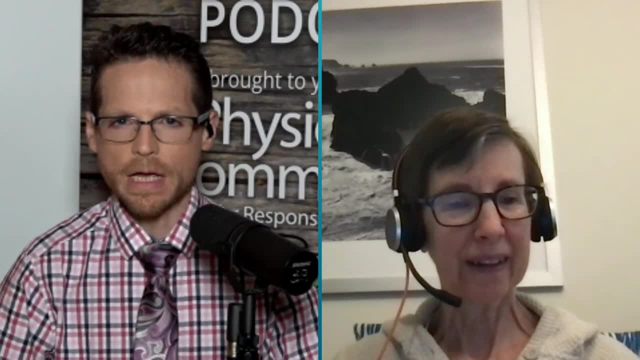 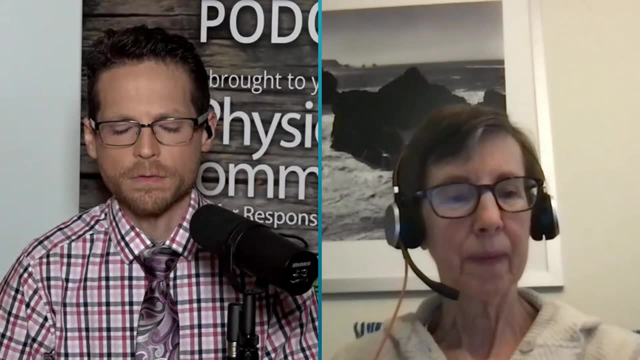 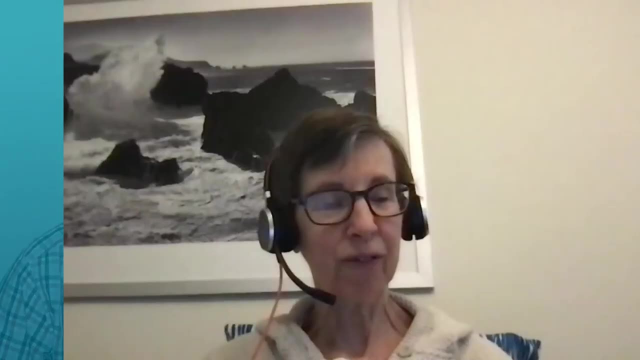 Um, as it stands now. uh, there is- I believe it's three days that people go through um, where they're coached up on how to do these classes. What was the training experience like for you? Um, it was amazing because PCRM had a grant at that point and they paid for us to fly. 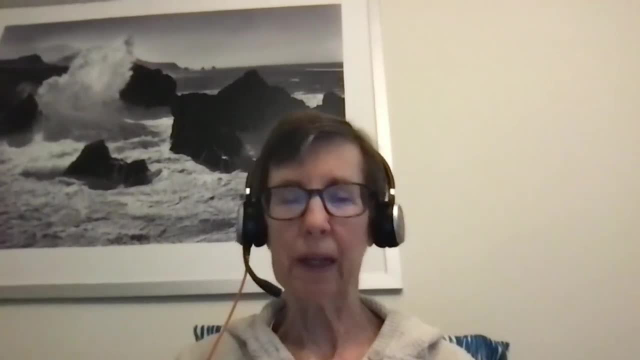 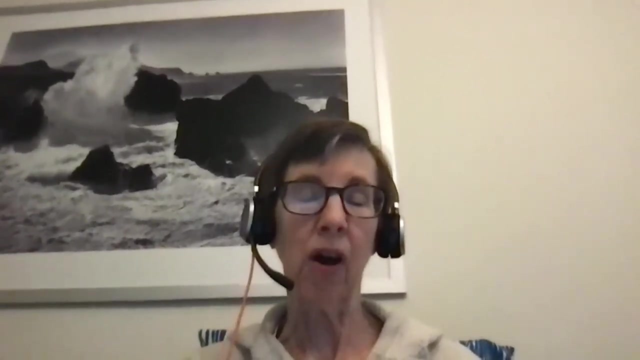 to DC for this three days, three, four days it was- And um yeah, we got to observe one real class being taught in person, And then we went through each of the lessons. There was only the cancer project curriculum at that time And it was called the cancer project. It wasn't called. 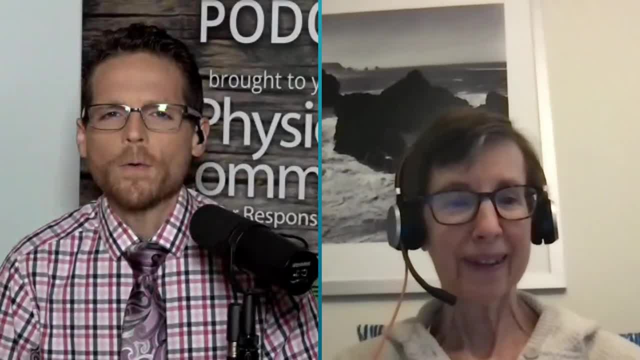 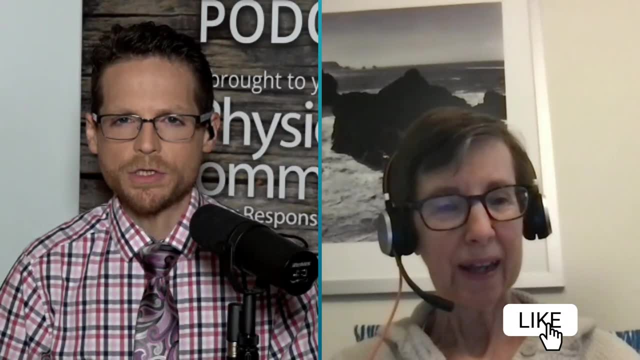 food for life. So you get your food for life- instructor credentials- Um. and eventually you begin to teach Um. and then you get your food for life- instructor credentials- Um. and eventually you begin to teach your first class. Do you remember teaching your first class? Were there. 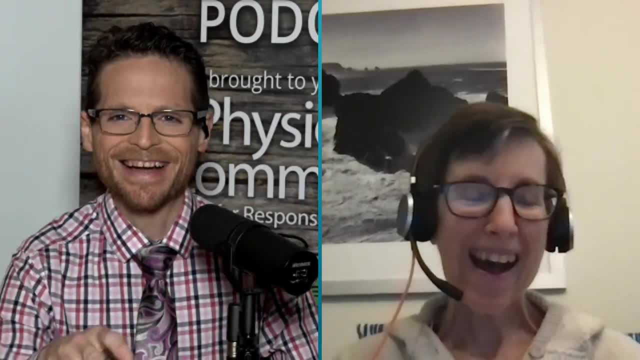 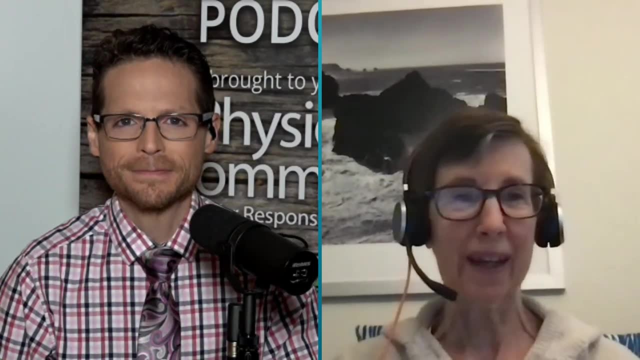 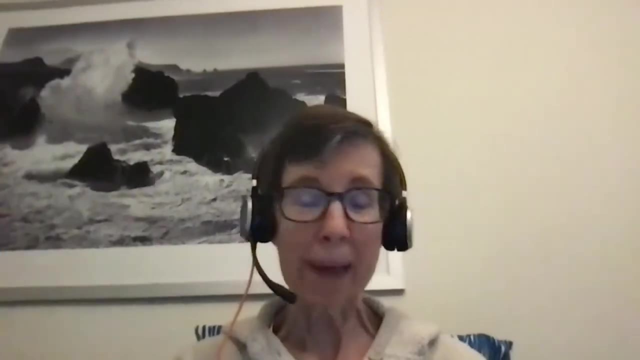 any jitters that you had? Oh heavens, Yes. Um, I was really fortunate. Uh, I went to the hospital where my husband was on staff and I talked to their um community liaison people and they were open at that point. PCRM paid for everything, So they didn't have to put up any money and I was 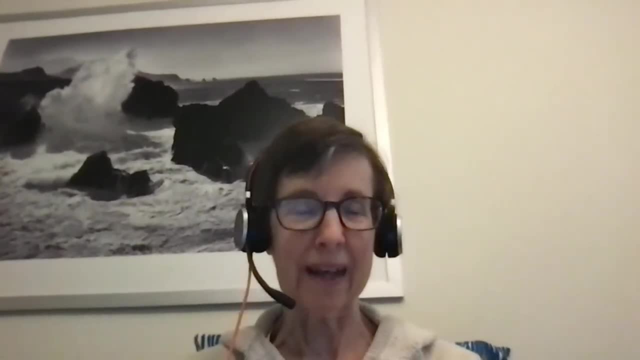 willing to teach. So they were fine, Go ahead and try it out. And so, Um, we got a classroom and it was on the hospital campus at that point, And I, uh, talked to the people at the newspaper. They put an article in and the first class was full within, you know. 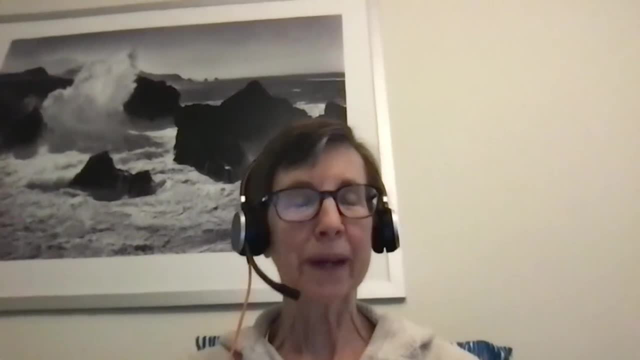 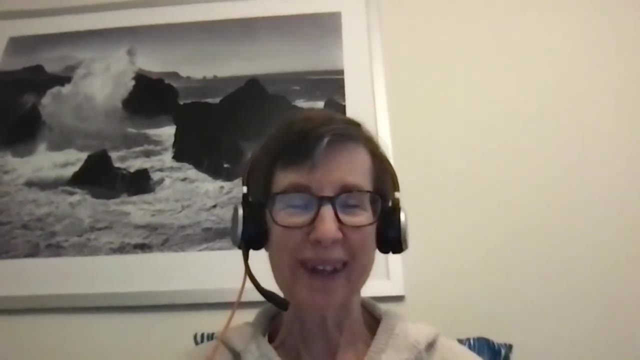 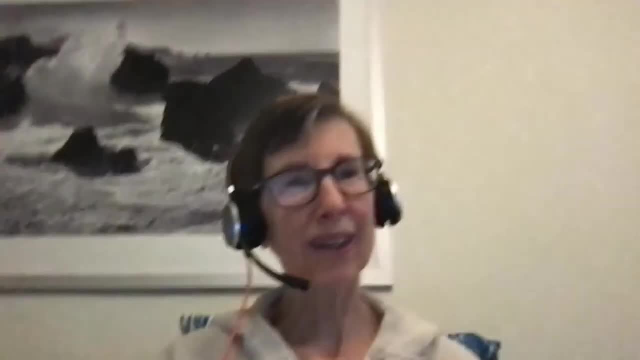 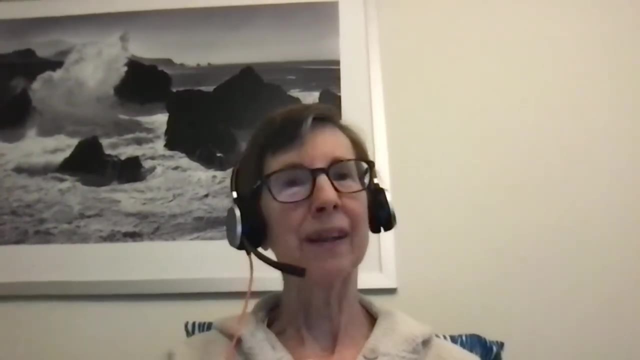 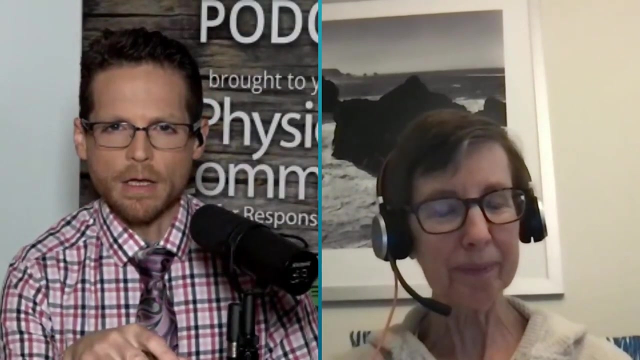 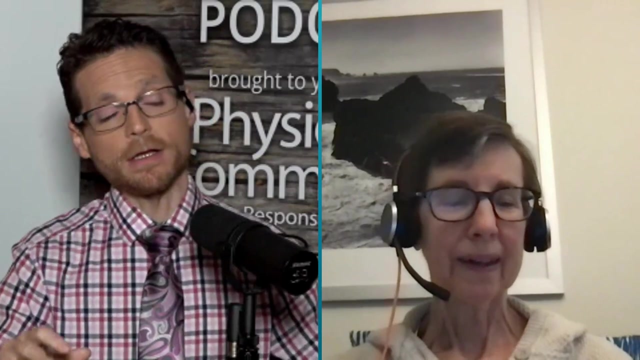 before And uh, but teaching it with the videos with uh Neil and having the curriculum kind of spelled out, um, it was really pretty easy, Okay. So to me it seems like you kind of went above and beyond what a typical person would do on their first time out, Like I would think that. 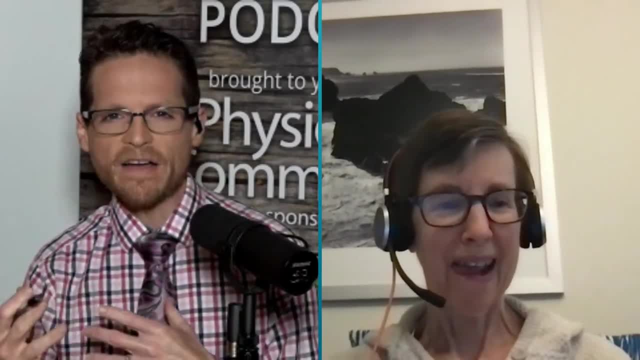 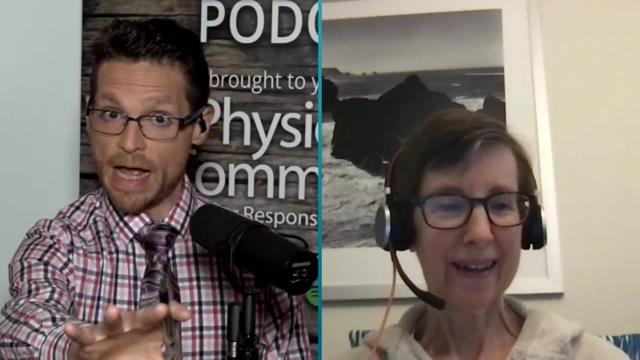 initially you're just, you know you're. you're looking to have maybe five people in that class- Maybe there's some friends And family filling up some of those chairs. but you go straight to the hospital and beyond that you reach out to the newspaper and say, Hey, this is what I have going on, Would you mind? 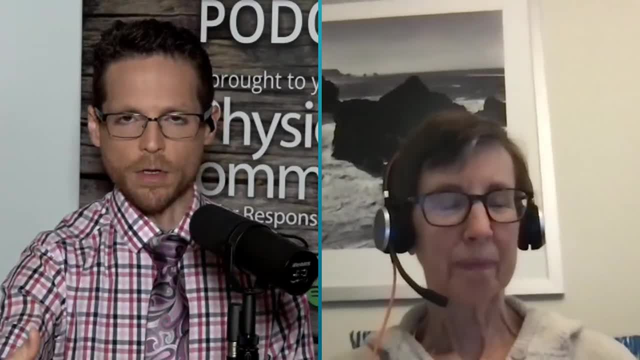 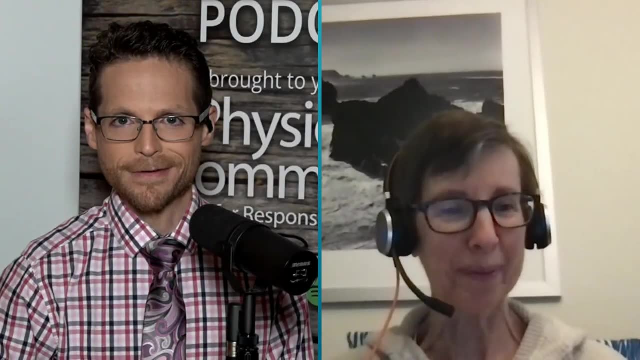 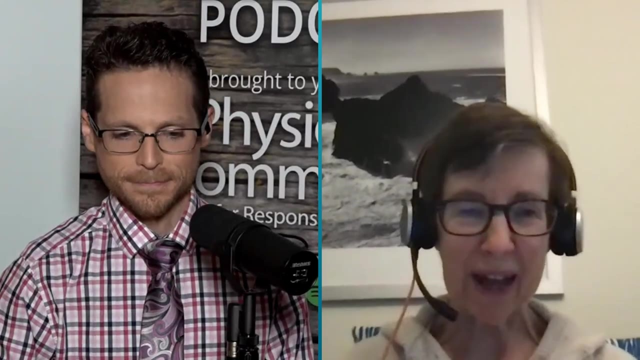 giving it a mention. Where did that motivation come from for you? Um well, I wanted it to reach as many as I could And so, yeah, we had 20 people. that was about my max at that point that I thought I was comfortable with the room and and the sample sizes and all that, And uh, yeah. 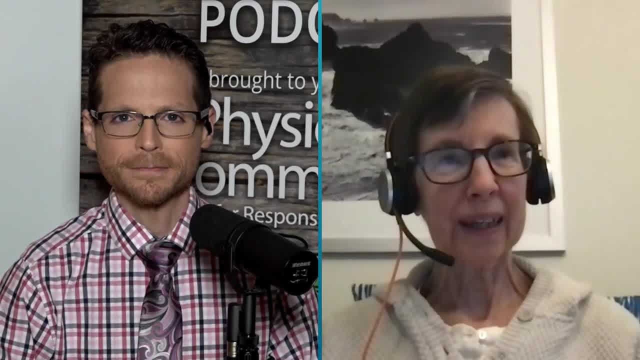 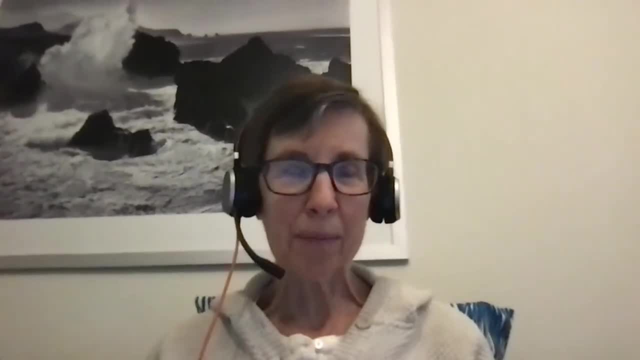 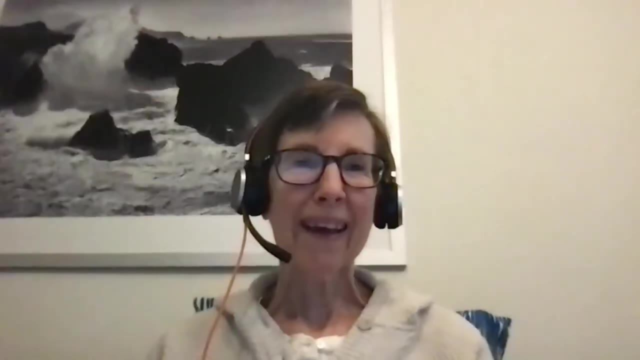 so. and then you know after that, um, I had waiting lists And so public publicity was not something I really had to worry about. Um I, I don't you know. I'm not much help to other instructors because I think the climate is different now. I think there's a lot more. 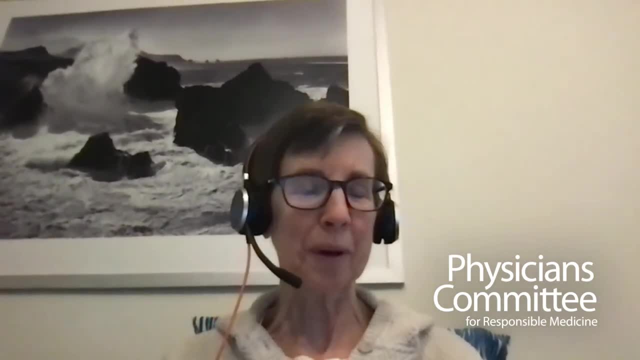 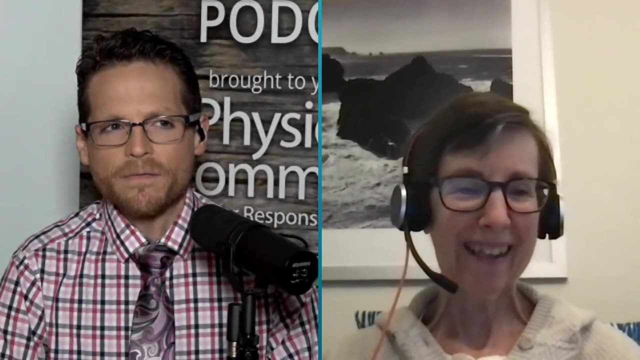 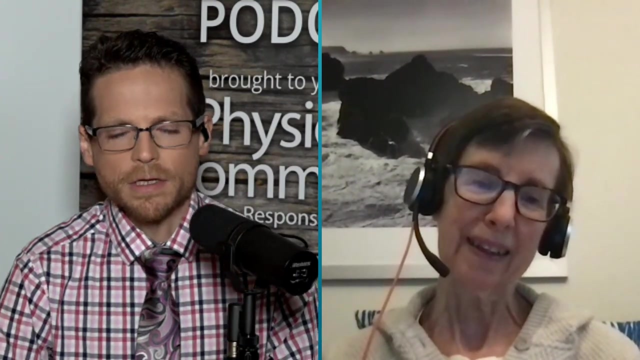 options out there for people, And so you're in a real competitive kind of place compared to what I was. Yeah, Well, I would say that, but I think that the the fundamentals are there. as as far as that drive to just get going, And it seemed to me like you didn't dip your toes in the water, You just 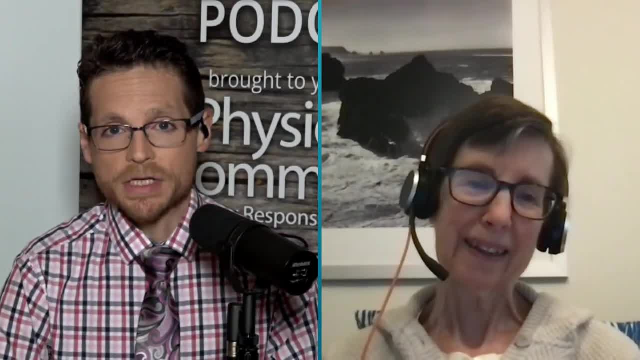 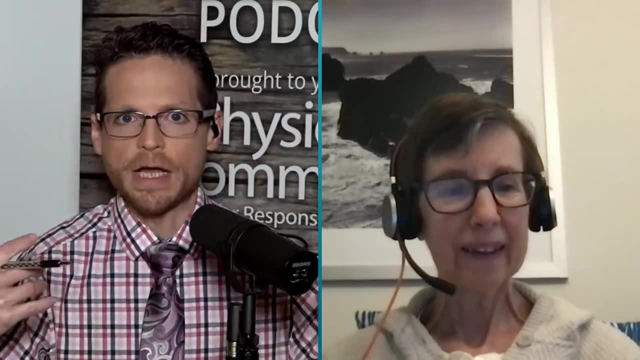 kind of pinched your nose and jumped right into the deep end and just got off and running. And I think that for food for life, and certainly in my experiences in media as well, is like when you just decide to do it and you push all the chips into the middle of the table. you go all in. 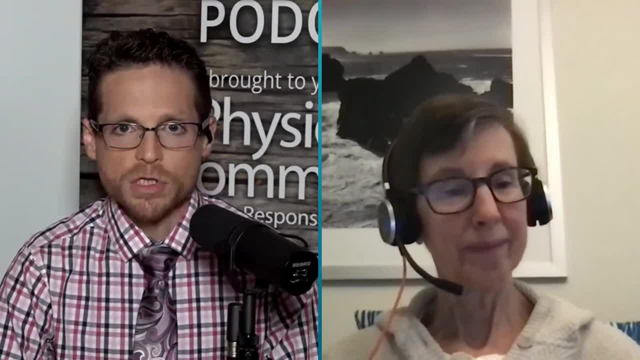 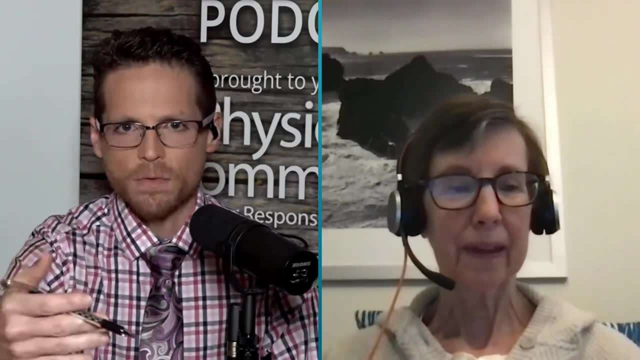 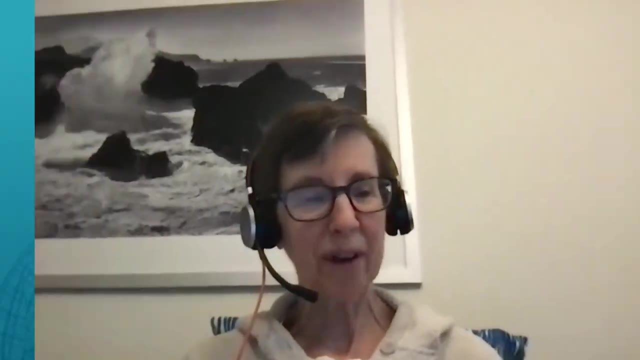 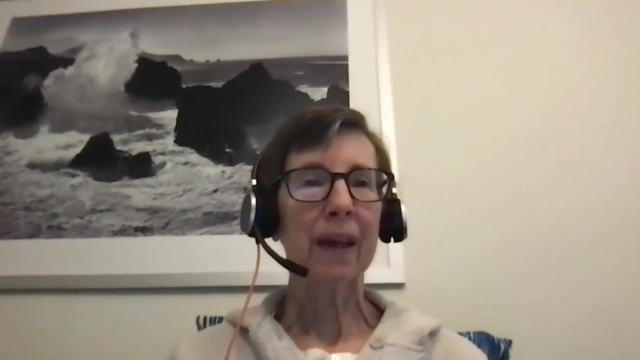 things just inevitably seem to work. Oh right, I mean, it's such a needed thing and it's so different from other things that are out there. I've gone to other cooking classes and, um, you know, the food for life programs make. 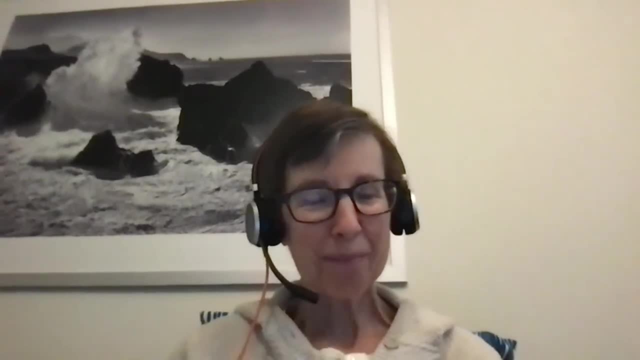 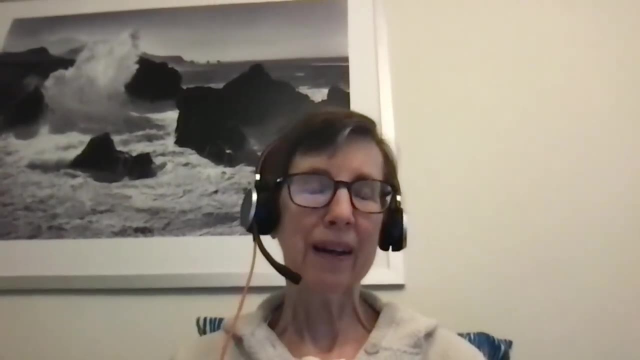 cooking easy. They don't make it complicated. People have said: Oh, I didn't know that, I didn't think I could do this, but you know, I found out I can. Um, so I, uh, I would not hesitate to do it. 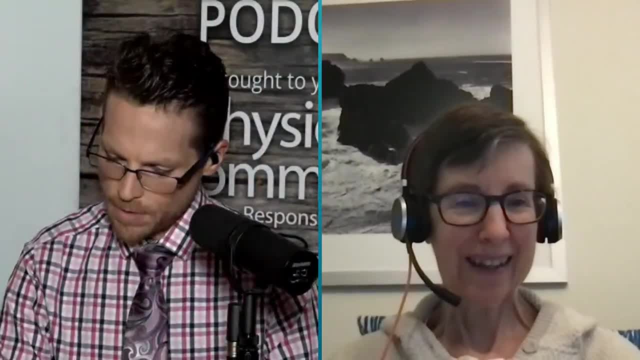 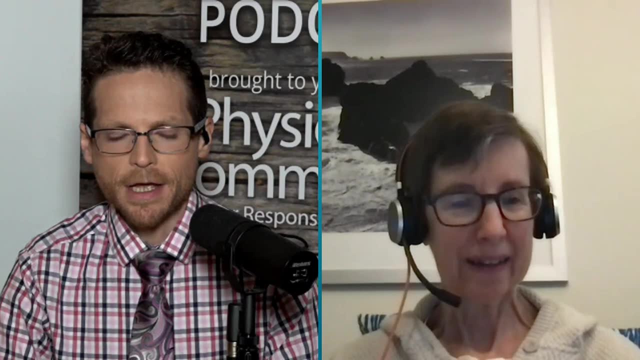 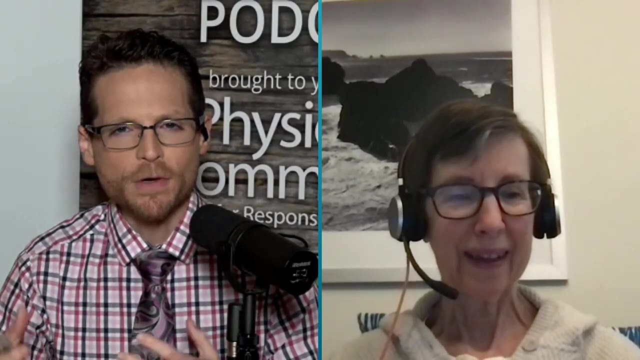 all over again. So this is uh all the way back in 2005,. you go through, uh, the training. Um, a lot of years have passed since then And now, who are some of the more memorable students that you've had throughout the years? Are there one or two that really stand out to you? 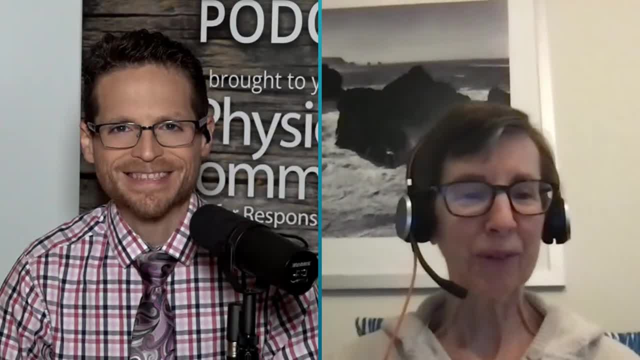 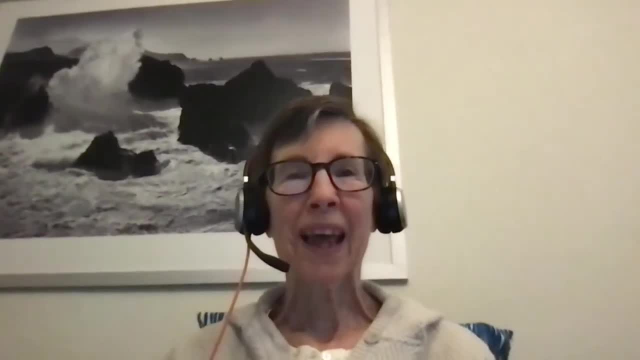 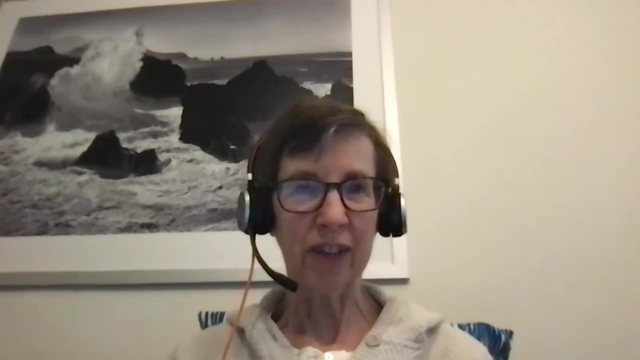 Well, you know, um, yes, there is one who really stands out. Her name is- and she wouldn't care if I told you her name- Her name is Edna, And when she took my class she was 82 years old. She changed her diet. 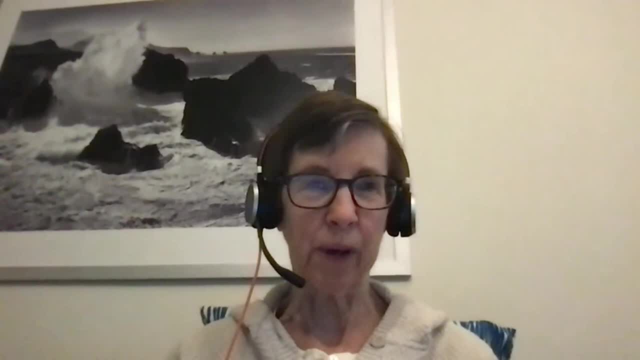 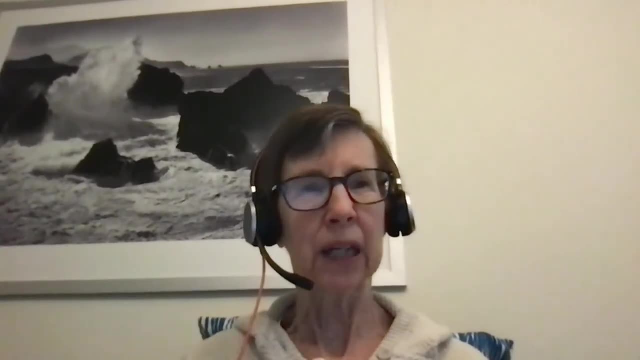 She said she felt better, as good as she had, when she was 40. And then, not only that, she was um, living in a sort of retirement community area, Um, and she started having food is fun classes at her house, teaching plant-based cooking. 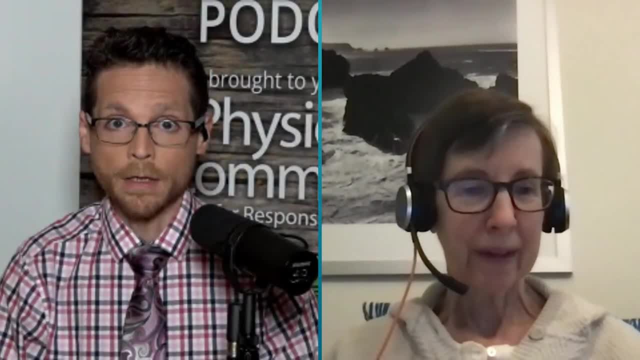 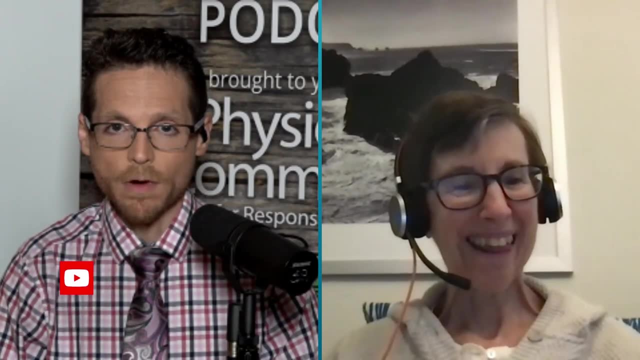 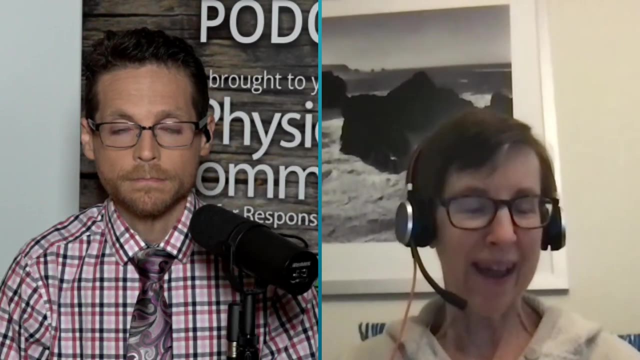 to her neighbors and her friends. Edna- Wow, That's phenomenal, She was amazing. What an inspiration. She wow, Yeah, Her husband died of cancer and she said: I don't want cancer in my house ever again And that was her motivation for taking the class. 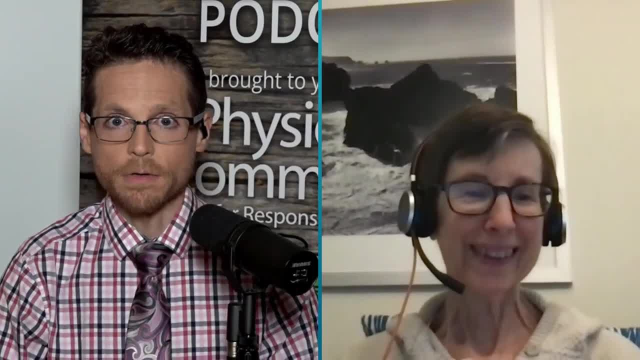 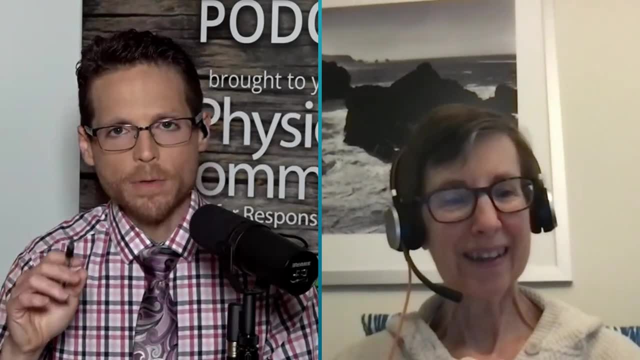 I would imagine that would definitely stick. stick with you as an instructor. I mean, how can you forget that story? My goodness gracious, That's. that's just incredible. Um, I'm noticing a theme with you, though. I was going to ask you what you get out of this. 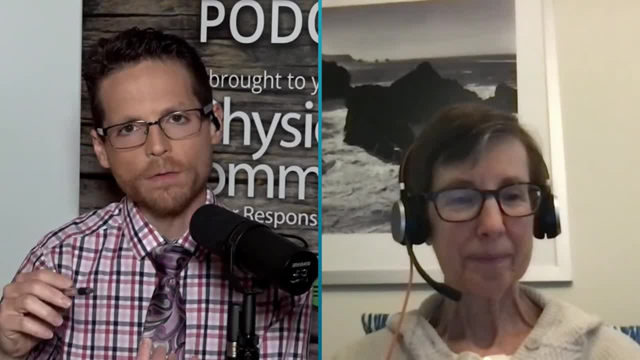 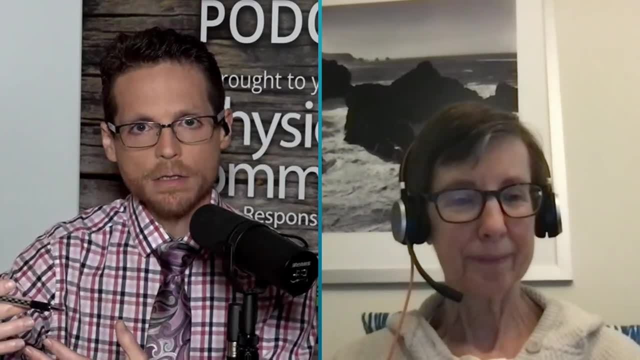 as an instructor. but it just hit me: It's like you went from being a nurse to being a therapist And then also, in addition to that, becoming an instructor, And so it seems to me like you just have this inherent drive that you want to help people. 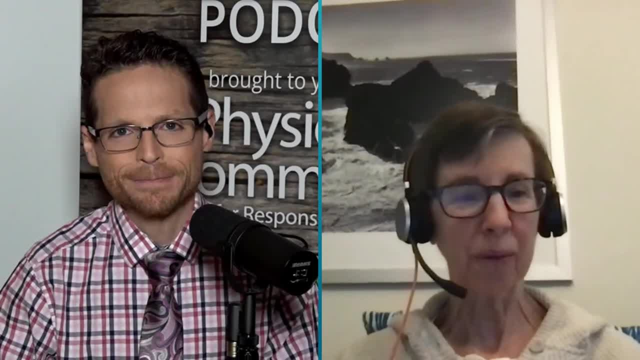 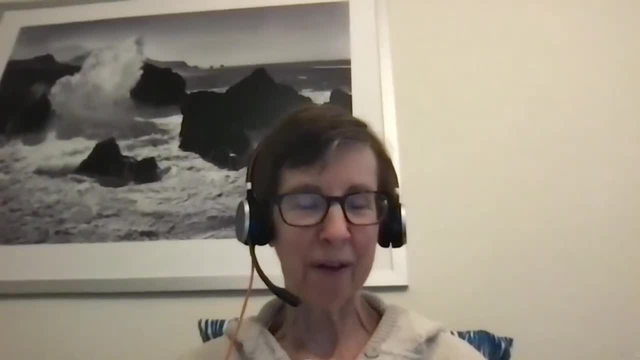 I guess you could say that Um, and it is a joy when you see people thrive. I mean even um, oh, I don't know. A few months ago I was sitting in the jacuzzi at the gym where I swim. 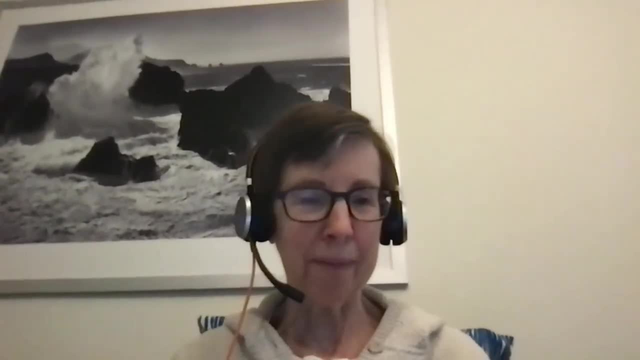 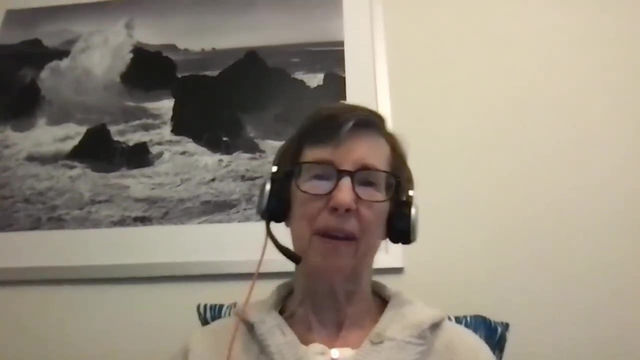 and this guy was sitting there and somehow we started talking about food and he said: oh yeah, my, my blood pressure's kind of borderline high and my doctor wants me to take medicine and I don't want to. And I said, well, have you tried Flexi? 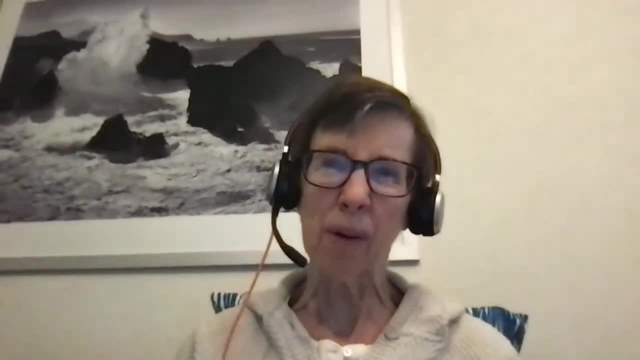 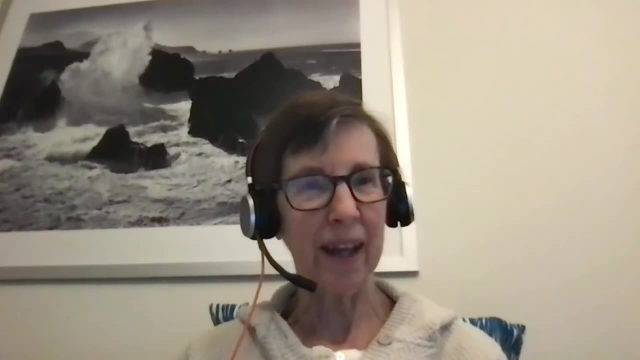 And a plant-based diet. And he said, well, I'm trying to eat more vegetables. So I said, well, try adding Flexi. And then I saw him a couple of months later and he said: you know, it worked. 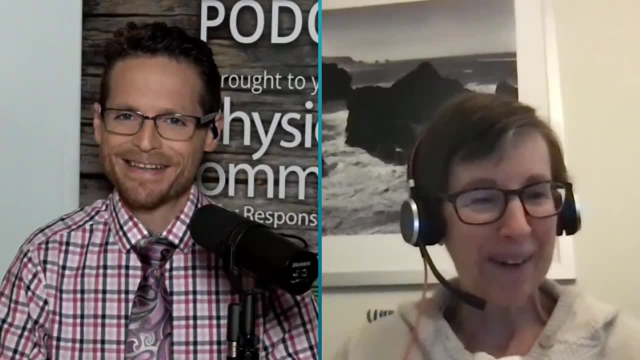 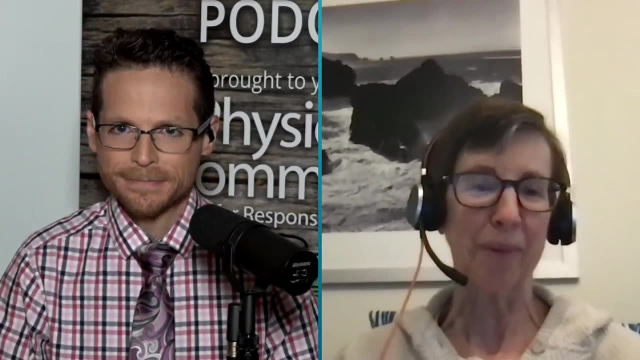 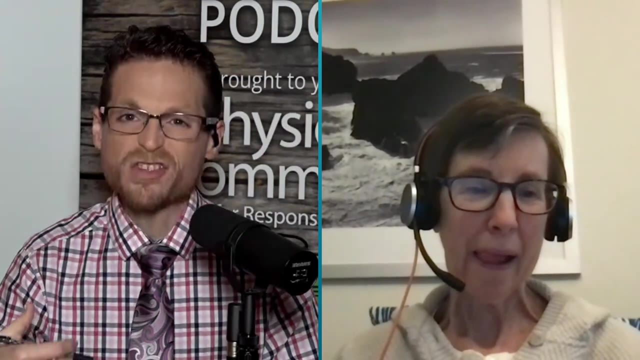 His blood pressure went down and he avoided. you know, he avoided medication. I mean that that is true. health is getting your health back, And I think that's what's important. So you hear stories like that, And then there's somebody who made 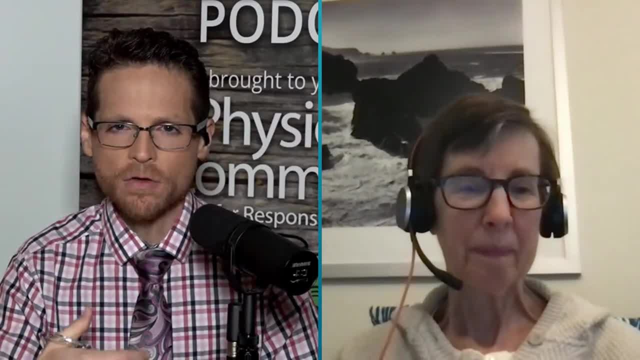 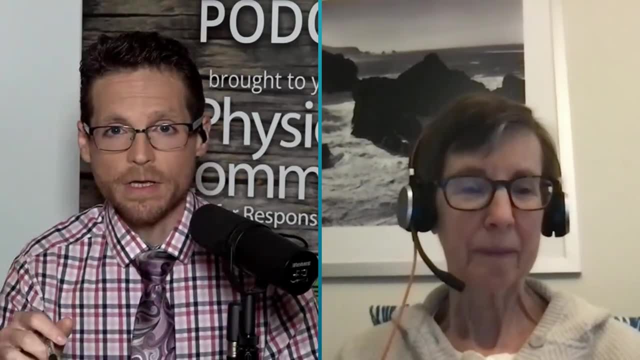 just be learning about a plant-based diet now, And you've been at this for so long- I mean since 1984 and then 1997, all in with the vegan diet, Jean, I'm going to ask you to look into. 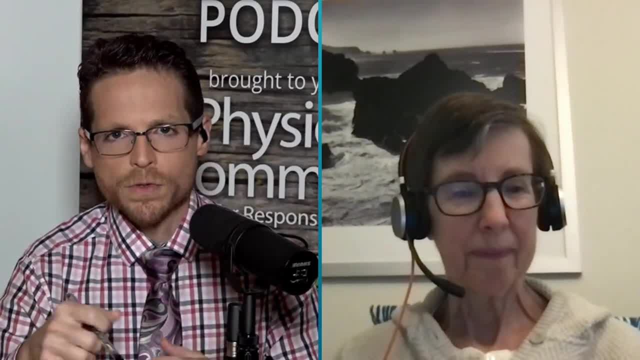 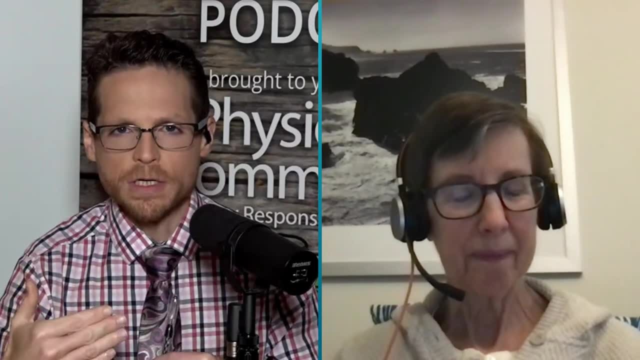 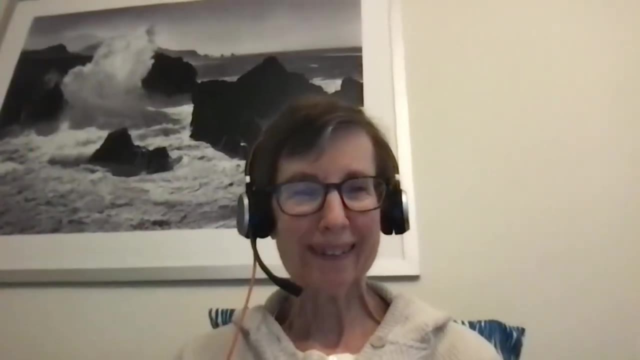 your crystal ball and look 20 years down the road for those new vegans. If they stay exclusively plant-based for the next two decades, what do you see in terms of their health? Oh, they will avoid being part of the health, the sick care system that we have. That is major, If you can stay. 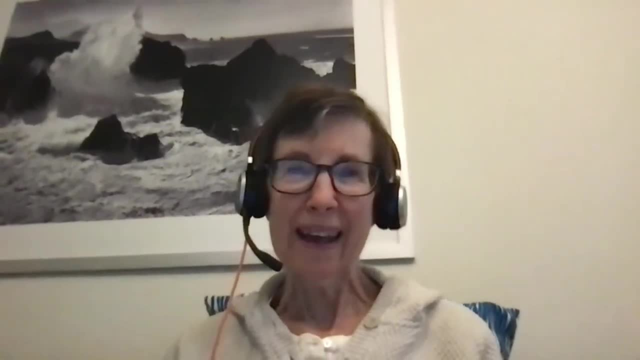 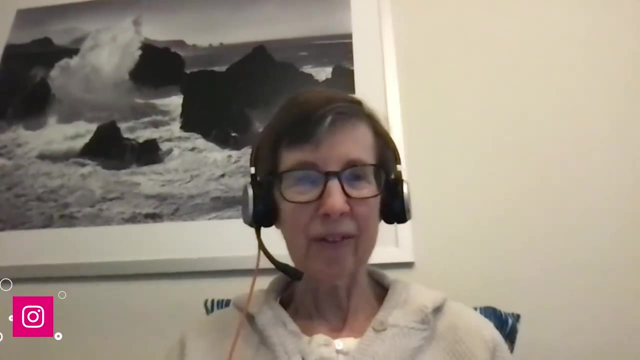 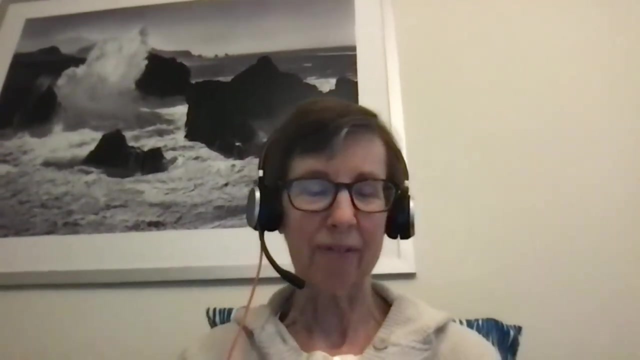 out of the doctor's office- that's what I think- And you have energy and vigor and you can enjoy activities with your kids, your grandkids, I mean. you can be there for their graduations and all that. I mean it just makes life so much richer. And another thing, as we try to wrap, 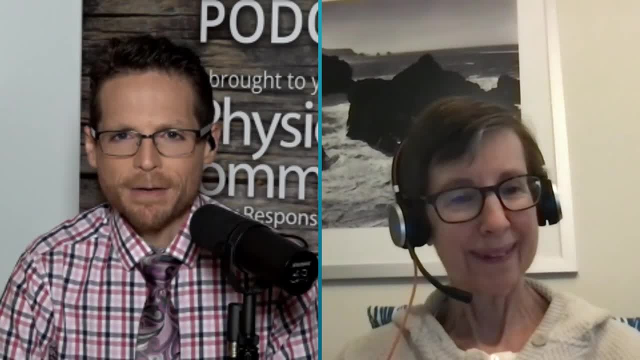 things up. I'm going to ask you a question. I'm going to ask you a question. I'm going to ask you up here. Jean, You've been really nice and generous with your time here, but I know for you a big driving factor for what it is that you're doing now is the connection between food. 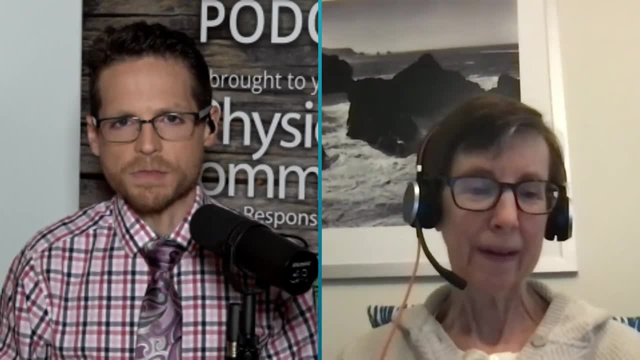 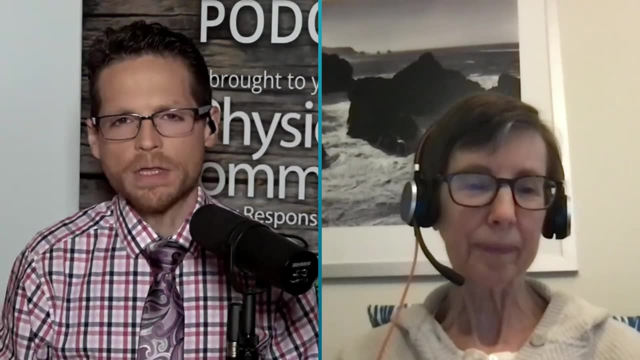 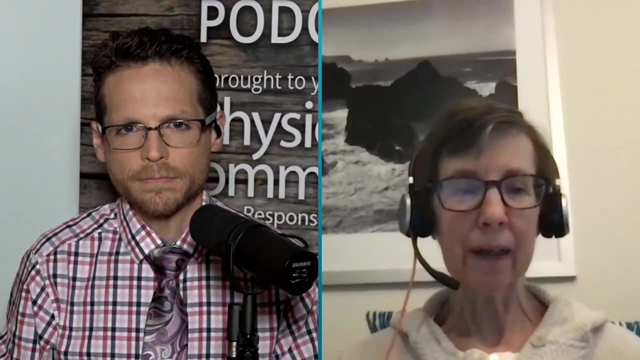 and climate. Obviously, that's something that's been on your radar for a long, long time. Like when we talk about food and climate, what do you think the average person is missing? Well, for one thing, most of the environmental organizations. 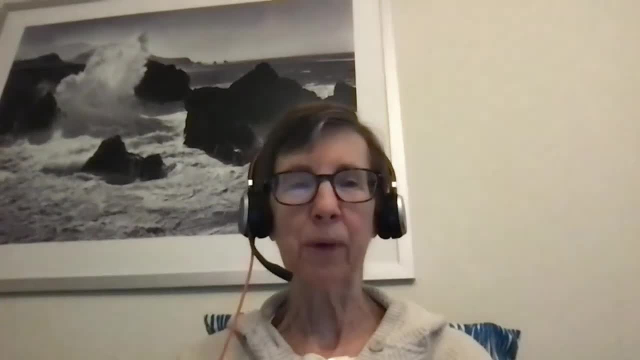 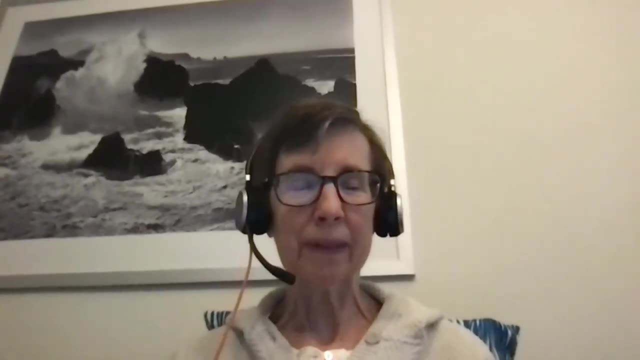 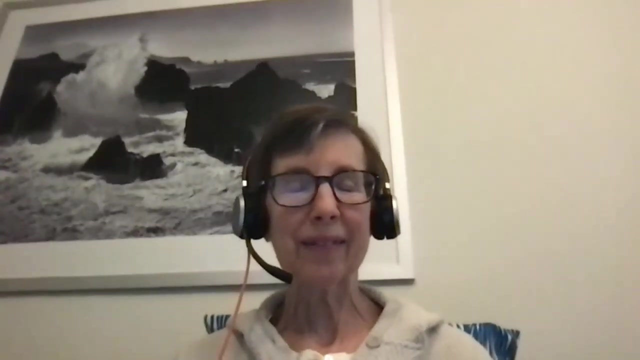 don't have it on their radar at all. So many people don't even think of a connection between what they eat and the climate. But the amount of land, water and other resources that growing animals for food takes is tremendous, And the cost, and all the forests that get chopped down. 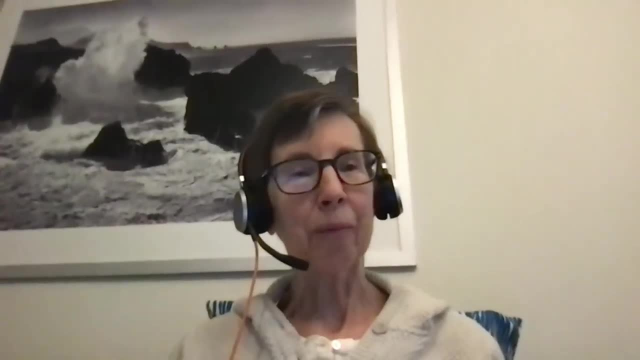 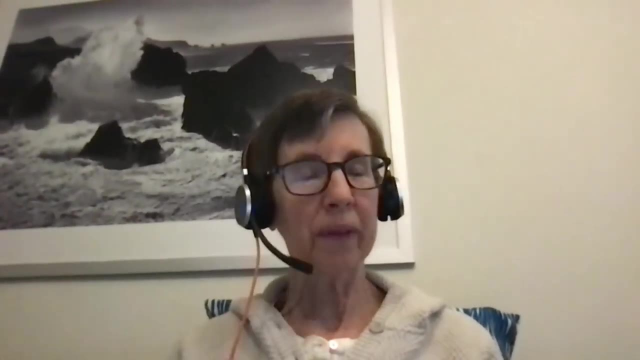 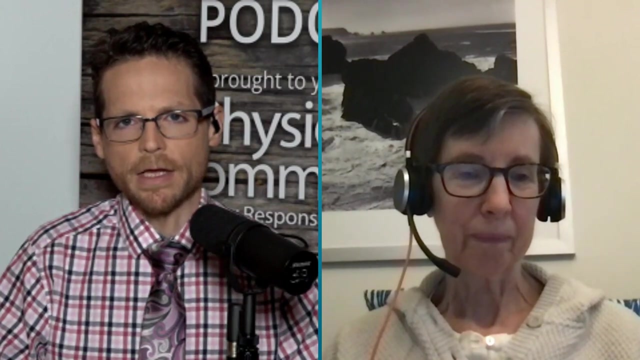 for grazing lands, and it just goes on and on. Whereas plant-based diets: we could feed everybody On this planet with enough food on a plant-based diet, And you're working tirelessly now to really educate people about that connection as well. 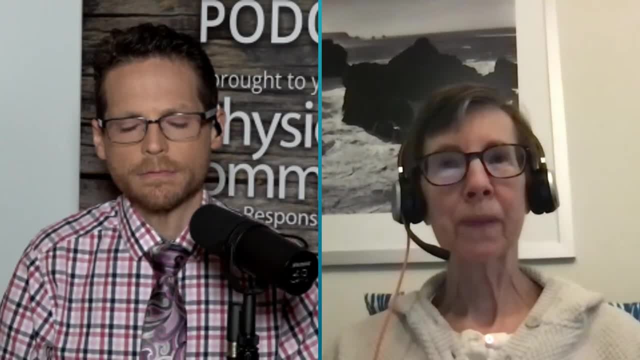 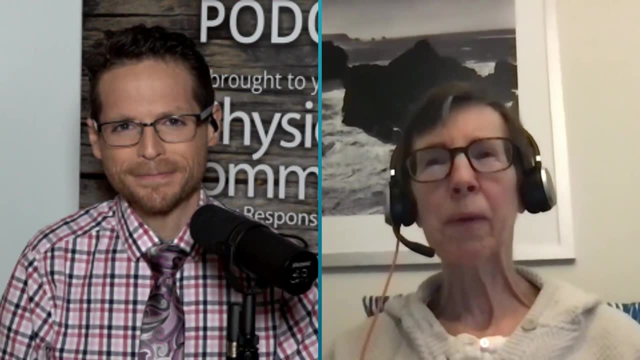 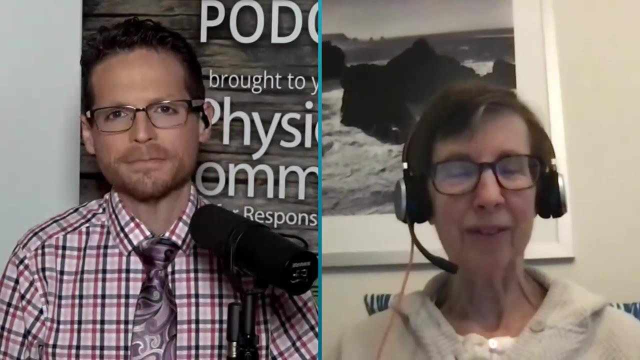 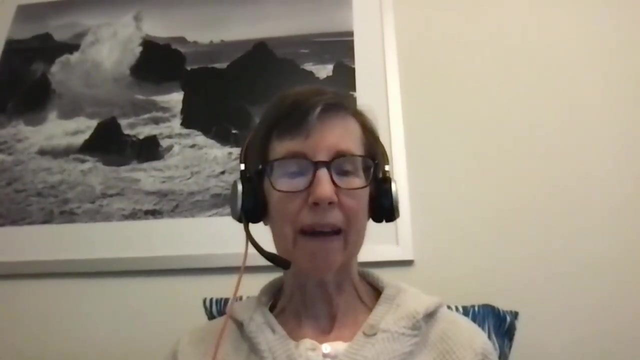 How is your message being received? Well, for the most part, yeah, for the most part. people are comfortable when you talk about stopping using fossil fuels, but they don't realize the impact of food And so, yeah, it is a challenge to get more people to see that. But, like PCRM's climate summit, 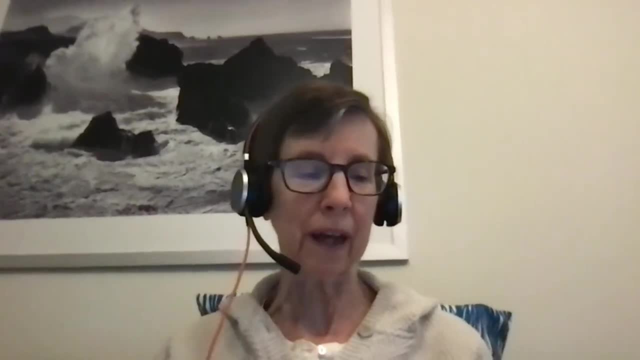 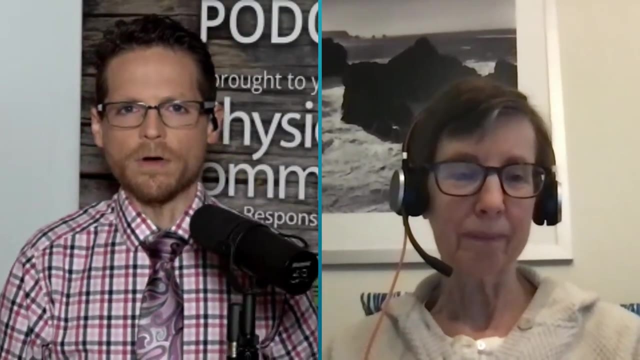 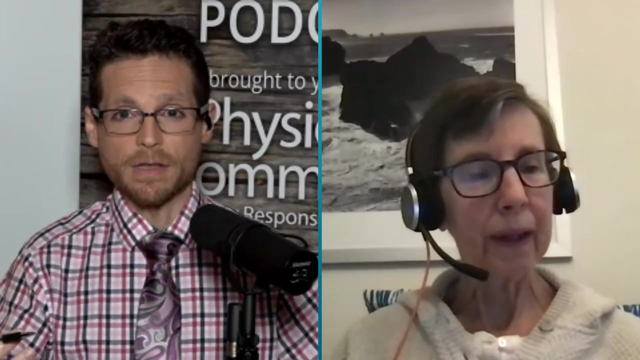 there are a lot of things happening now, especially that I think people will start to wake up a little bit. And what are some of the projects that you're involved with now to really try to help educate people about that connection, that trip to the drive-thru, that trip to the? 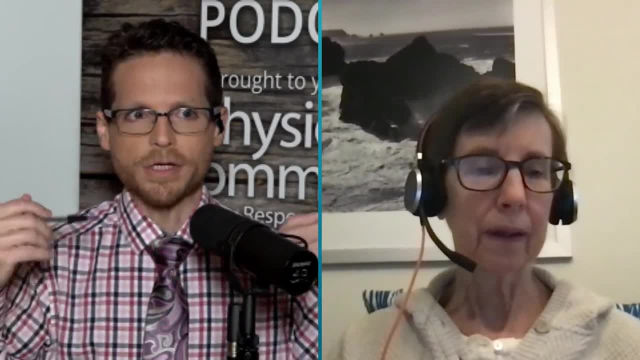 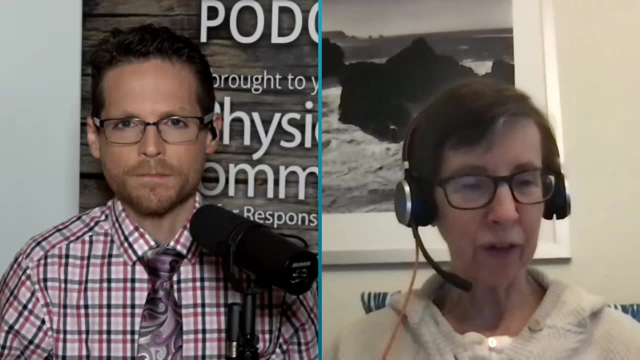 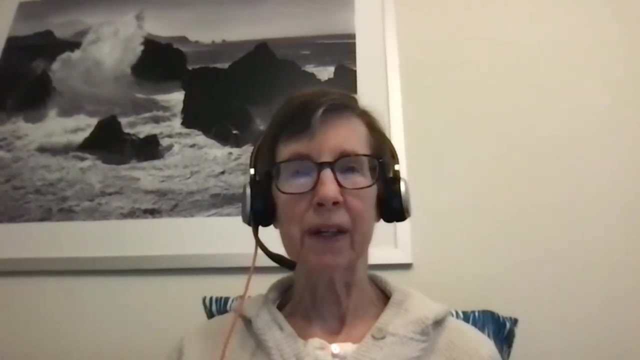 drive-thru. Well, I think the climate summit is so much more detrimental than just to your own health, Right, right, Well, I've been involved in a climate action group that's part of a Buddhist organization And we put on a day-long online event during COVID about the climate and what. 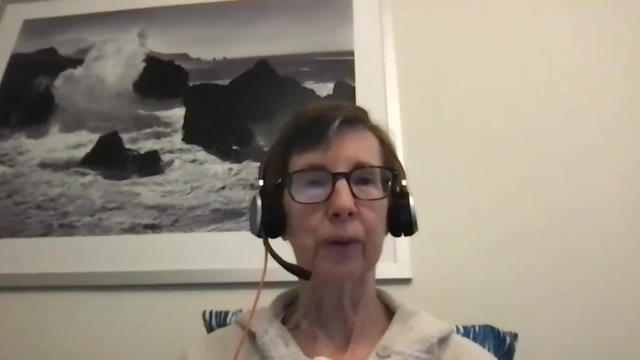 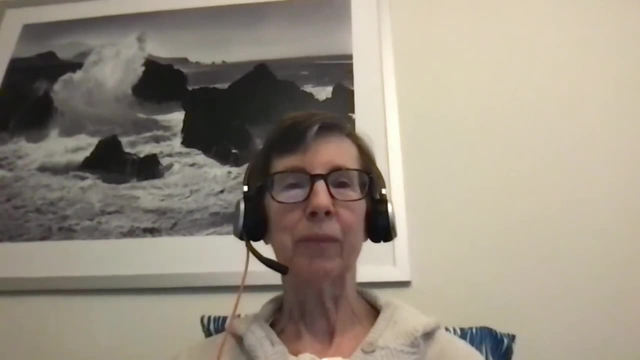 people can do, And I did a whole thing on food for that, And I'm also involved with an organization called Climate Healers. You can find them online, climatehealersorg. They promote a vegan world by 2026.. So they're. 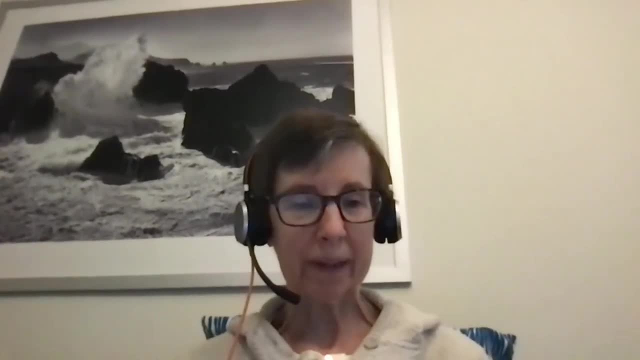 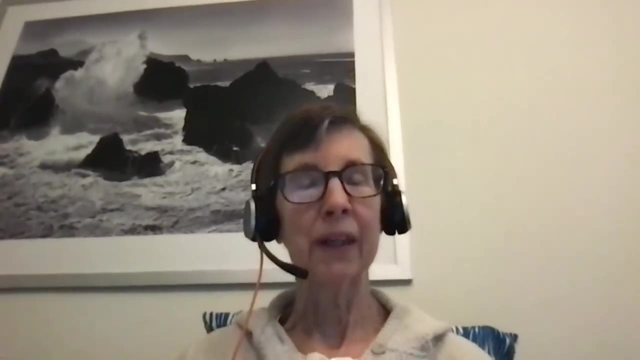 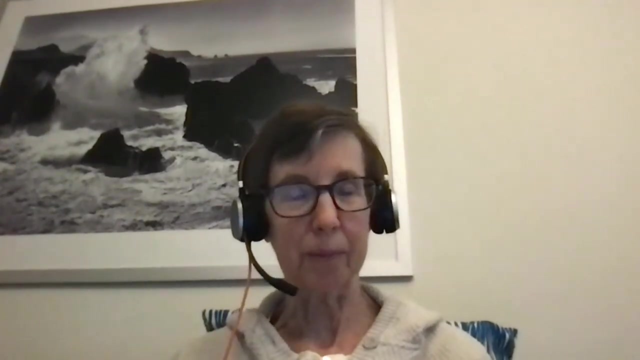 very audacious as far as their goals, But the thing is we don't have a lot of time left, And so I believe we do have to get audacious about what we're helping people to see the connections, And I truly believe people want this world to be healthy for their children and 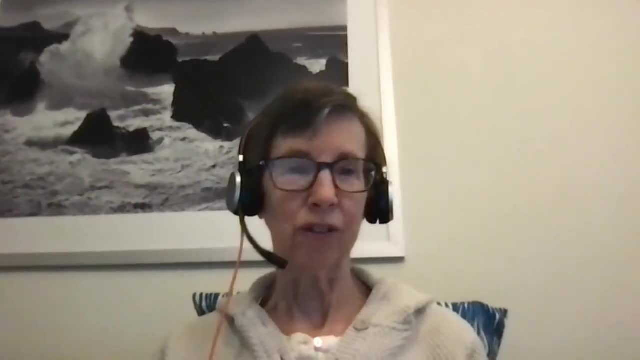 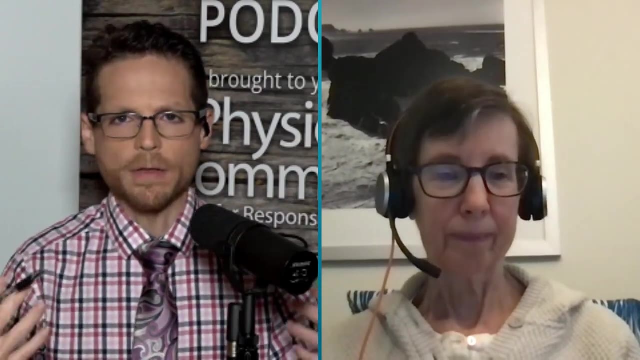 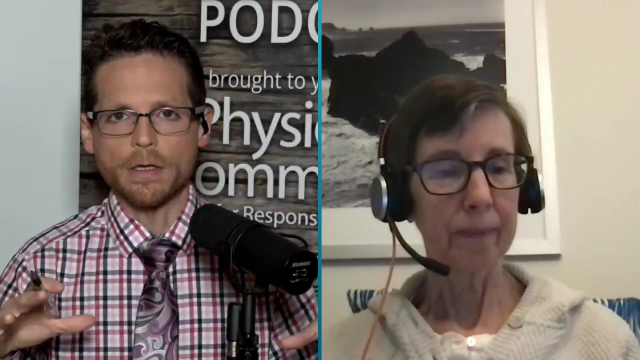 grandchildren And it's really not that hard to change your diet. And you know, the Food for Life program does a lot to educate people about the benefits of a plant-based diet And those do extend. Obviously, that program focuses on health, But the benefits